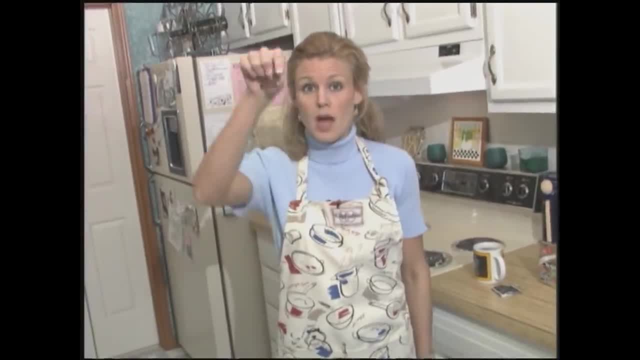 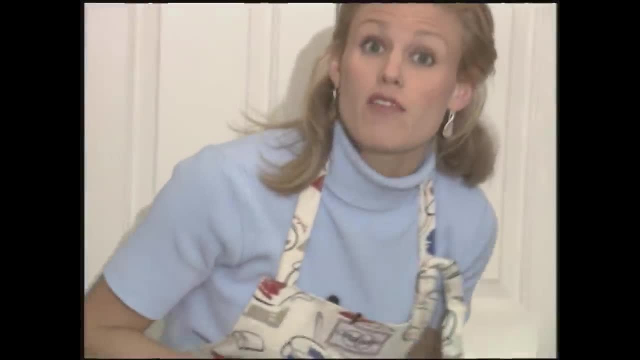 states of matter into three parts. The first part is the end of carbon. The second part is carbon dioxide. Now let's go back and see how you do that, Okay, okay, so we've got two groups: mixtures and solutions. Take salad dressing. Most salad dressing is made of oil. 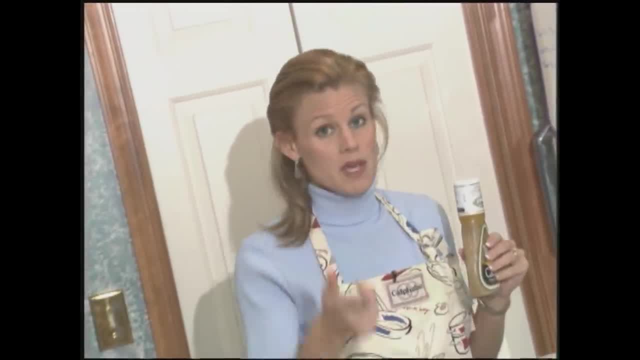 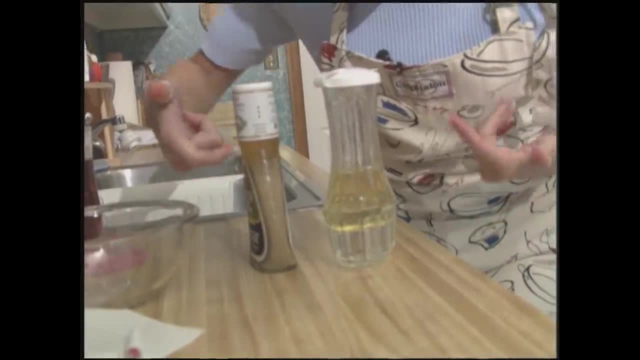 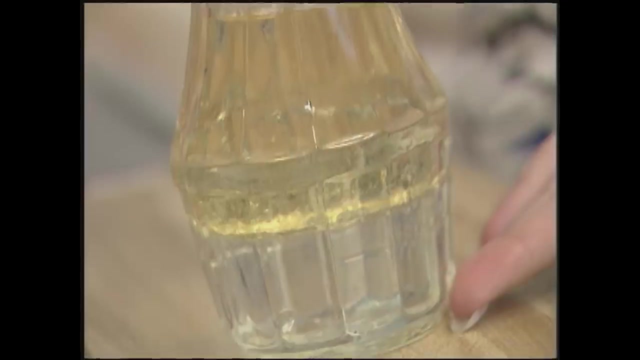 and vinegar, two liquids that are placed together but can be easily separated. If you let the salad dressing sit for a while, what happens? Well, take a look: The oil and vinegar separate. The oil is lighter, so it goes to the top. The vinegar is heavier, so it stays on the 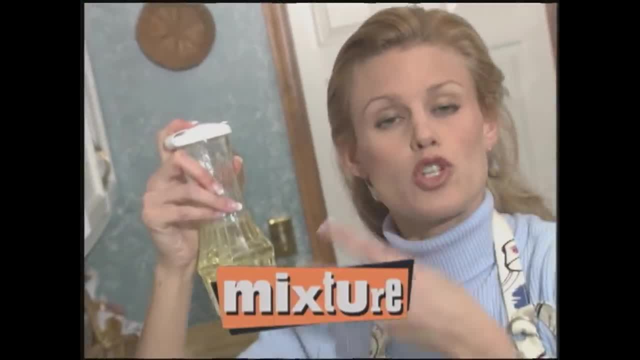 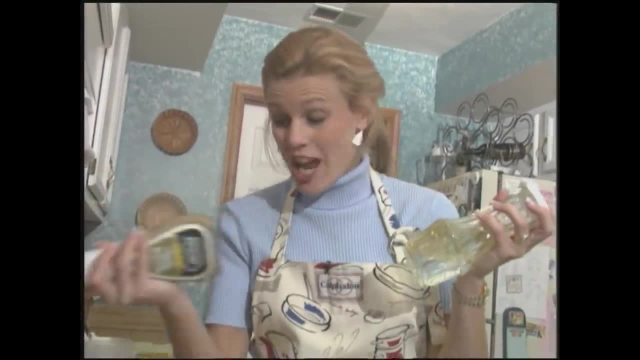 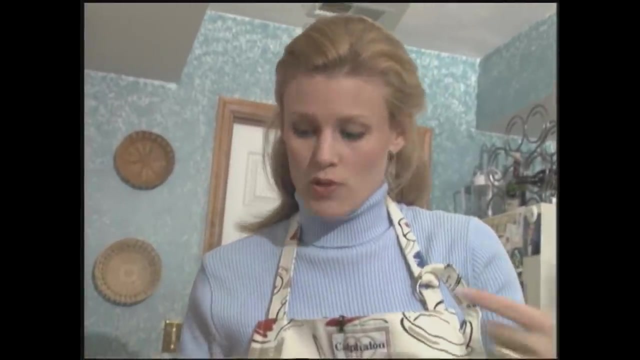 bottom. This is a great example of a mixture. These are two liquids that don't mix well together. That's why, when you have salad, you have to shake it up before you pour it on your salad. You don't just want all oil on your salad, You want to mix it up. So they 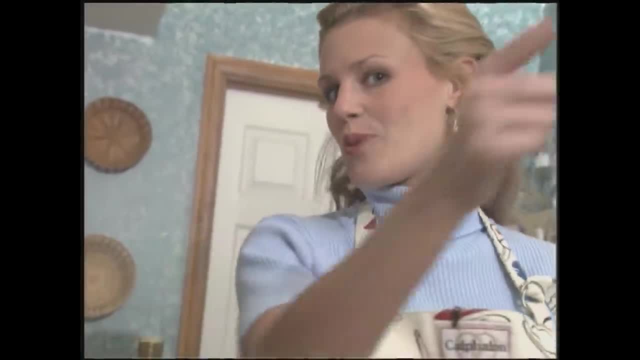 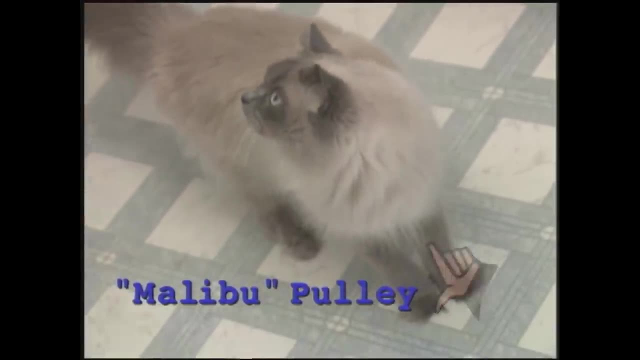 mix up for a little while, but then let them sit and guess what will happen? That oil will go right back up to the top. Go check your own refrigerator, You'll see what I mean. Get off the set We're trying to tape here. 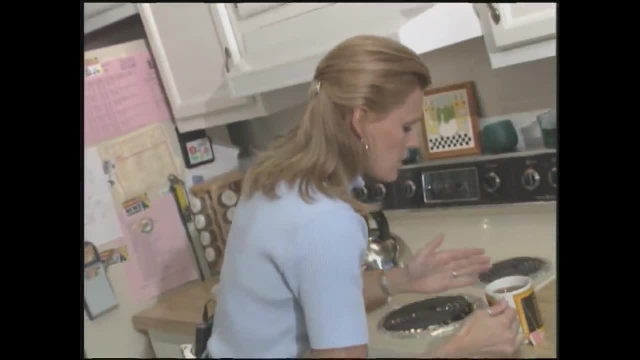 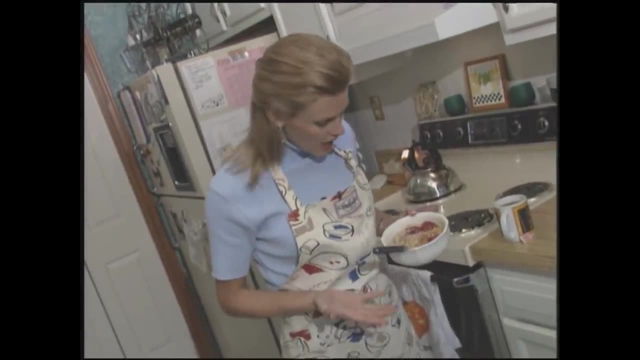 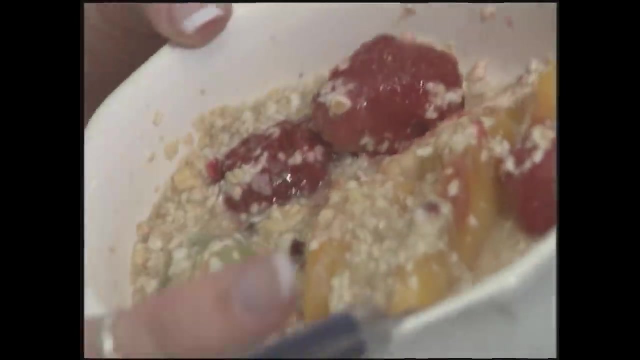 Here's another mixture for you. What about your breakfast cereal with some fruit? Here you go: oatmeal with fruit. This is a mixture because the fruit can be easily separated from the cereal. Just pull out the fruit if you don't want it, No problem, Easily separated. 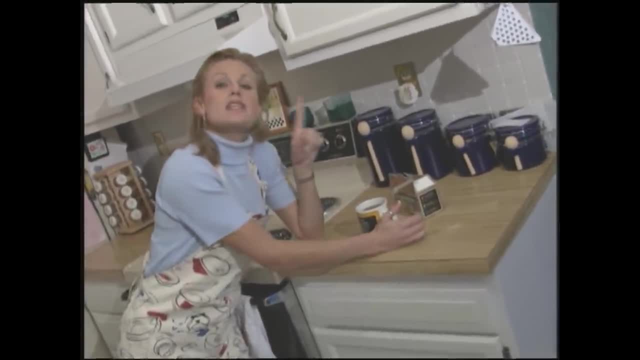 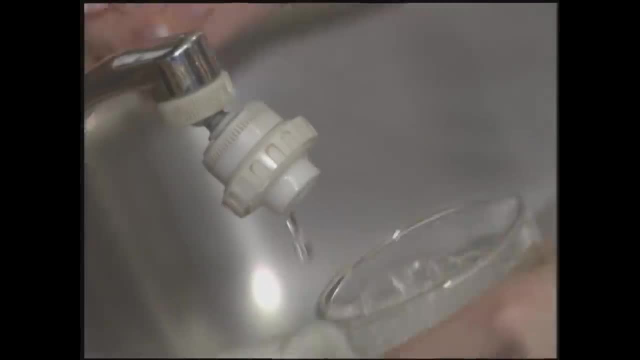 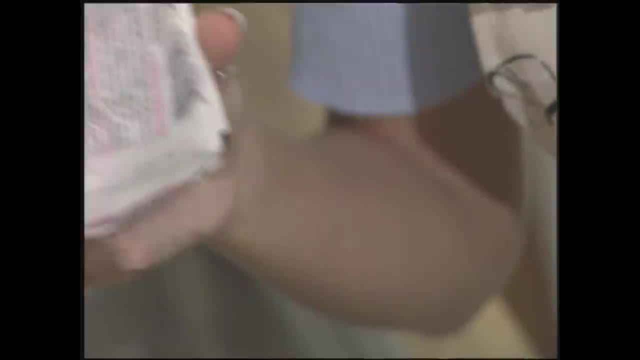 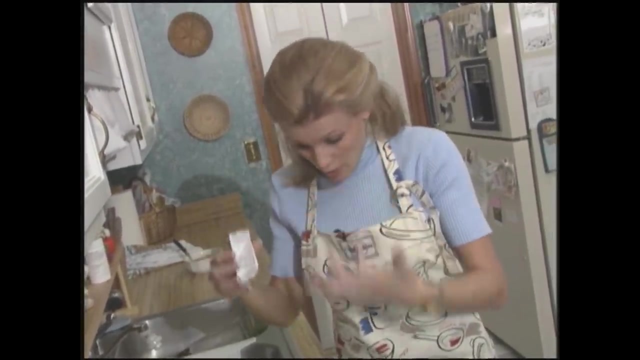 Here's an example of a solution. Take some water and powdered drink mix- Kool-Aid, Wyler's, whatever you got. Now, when you mix the powdered drink mix with the water, you have a mixture right: Two substances that are mixed together. 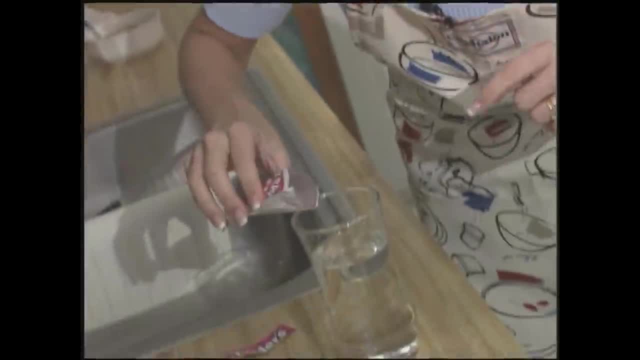 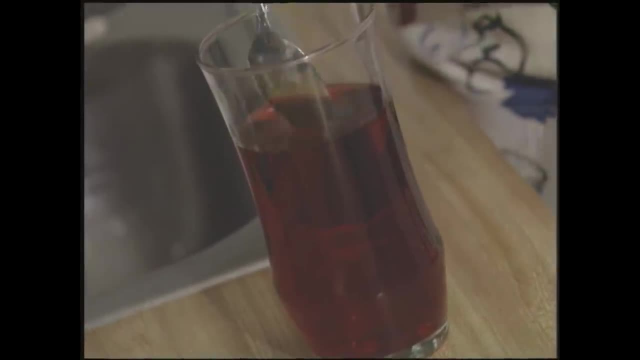 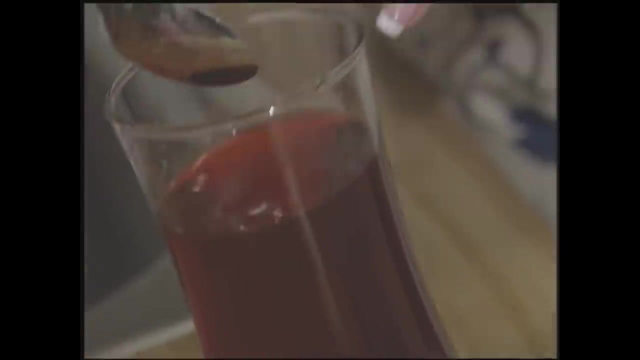 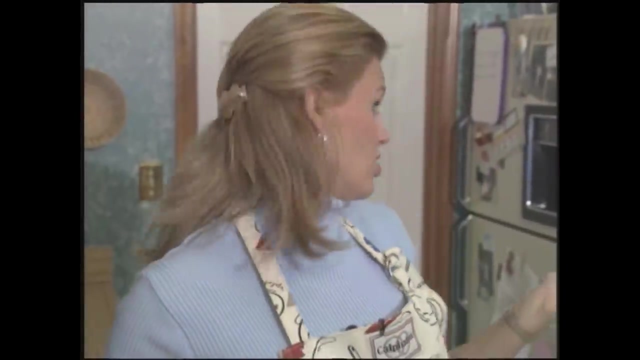 But this is a solution. Let me show you why. Watch what happens, Because the powder dissolves or spreads evenly throughout. this mixture is also a solution. There's really no way that we could separate the powder from the water Well, unless we had a lab or special equipment, which I 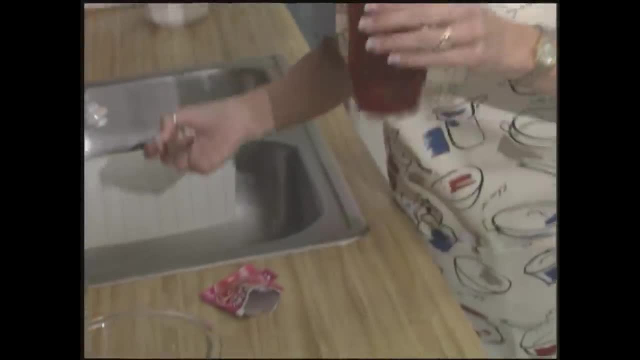 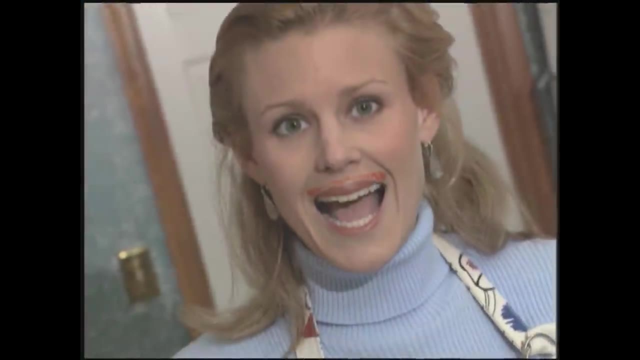 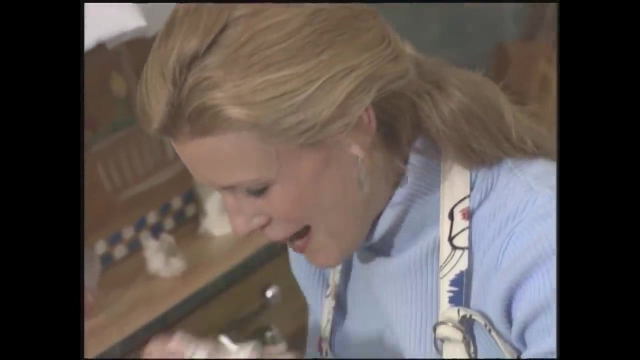 don't have in my kitchen. So the only thing we can really do with this solution is drink it and enjoy it. Man, I can't get this permanent cherry grin off my face. This stuff is permanent, So do you get it? All solutions are mixtures. 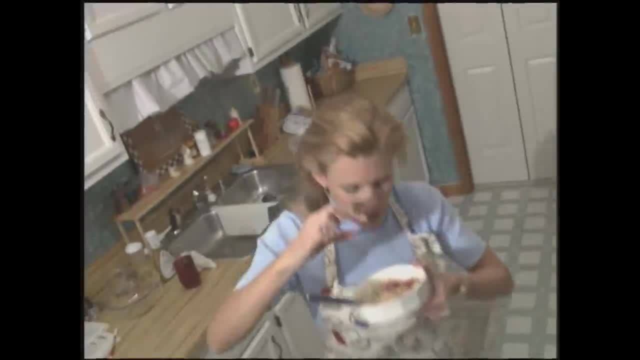 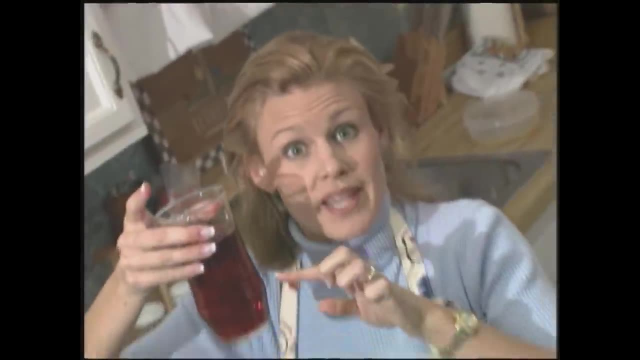 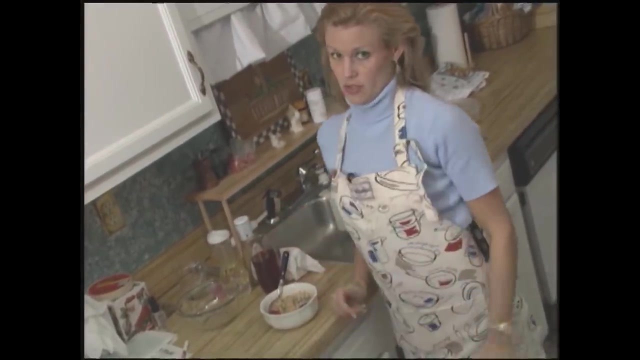 But not all mixtures are solutions. Here's my point. My fruit did not dissolve into my cereal like the cherry mix did in the water Solution and mixture- just a mixture, Not a solution. Now this is your last chance. I hope you've been paying attention. 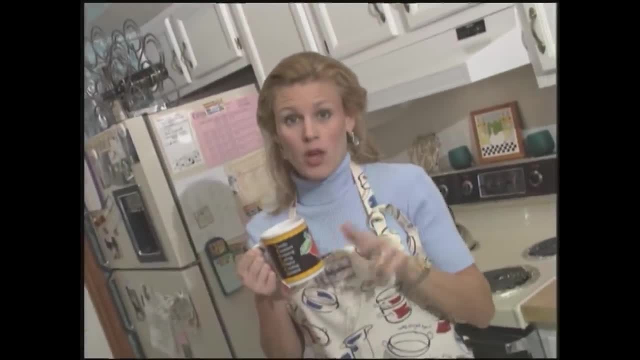 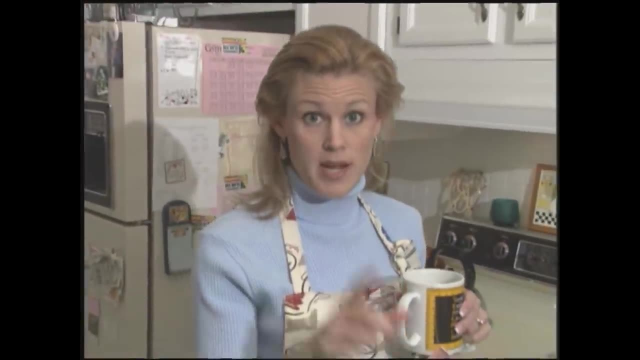 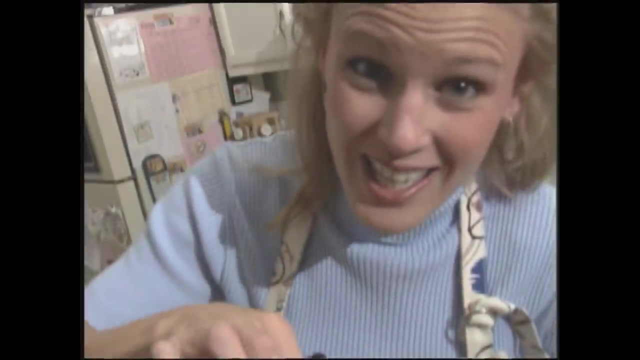 I sound just like a teacher, don't? I Remember mixtures can be easily separated without a laboratory or special equipment, And solutions are hard to separate because one substance is dissolved into another. My tea Solution. Hope you knew that Let's go meet a friend of mine. 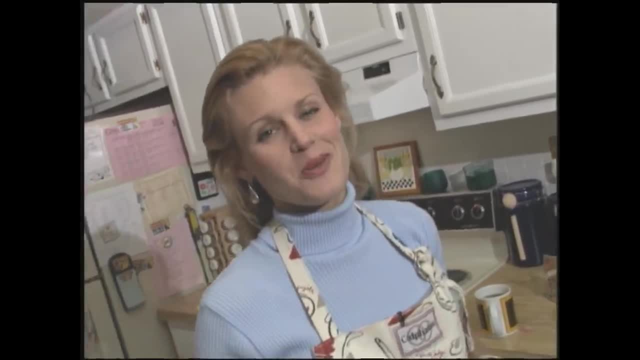 She's a doctor- Well, not the kind you'd want. I'm here with Dr McDaniel Now. doctor, can I call you Trish Sure? Okay, You are a doctor of. I'm a polymer chemist here. 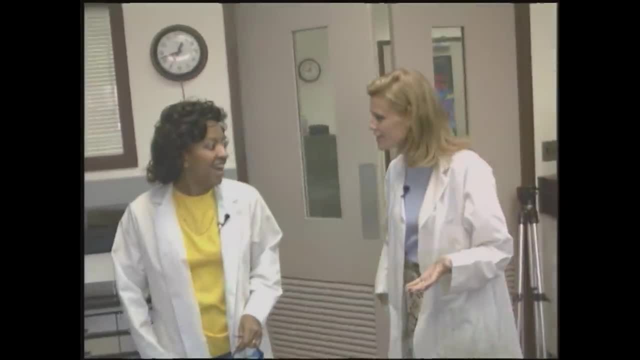 And we're here at NASA Langley Research Center And this is a synthesis lab that we're standing in. This is your lab, right? Yes, Oh, great, Great. So this is where I spend my days, Okay, And I see we've got these nifty little glasses here. 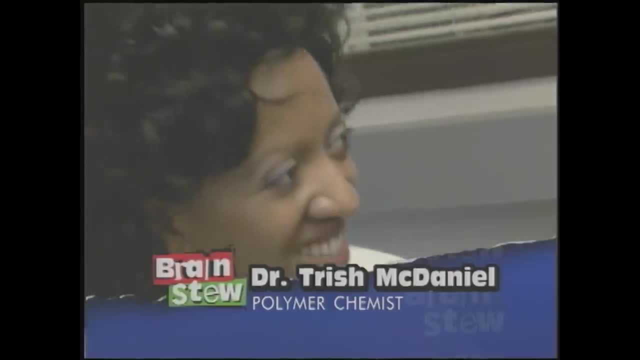 That's right. And whenever you're in a synthesis lab, we have some certain safety concerns, And number one is our eyes. Okay, So we always wear safety glasses, Okay, And I see we've got these nifty little glasses here. 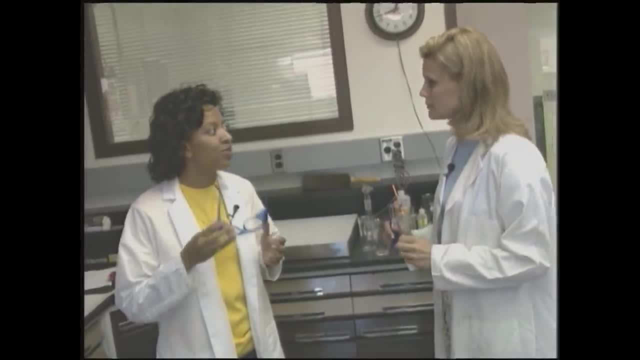 That's right. And whenever you're in a synthesis lab, we have some certain safety concerns, And number one is our eyes. Okay, So we always wear safety glasses. These are cool. I like the colors. Oh yeah, We had to do some. 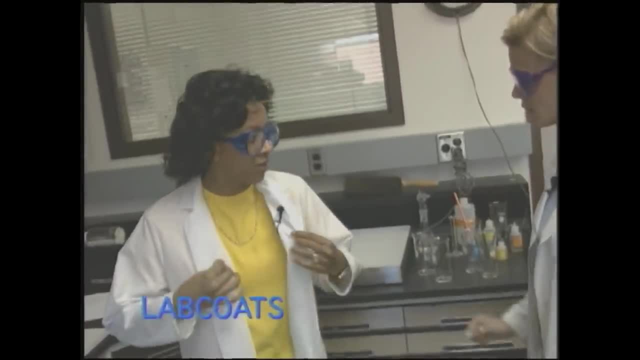 They're pretty hip in there, And another thing that we do is, whenever we're working with things, we like to wear lab coats, Yep, And gloves. Oh great, So you have some of those for me. Yes, Okay, Great. 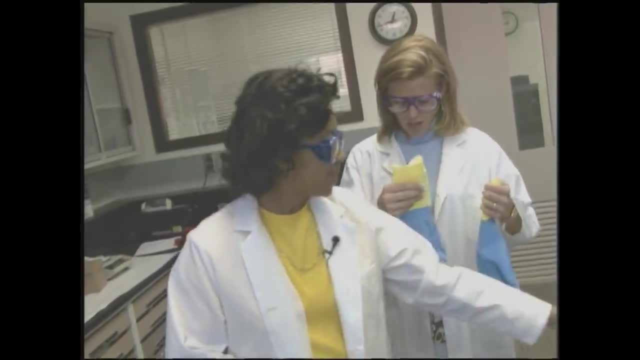 We're going to put on gloves as we do our different experiments. Okay, Now you know we've been. Oh, thank you. You know we've been talking about mixtures and solutions on the show. That's right, And you know you just were the perfect person to give us. 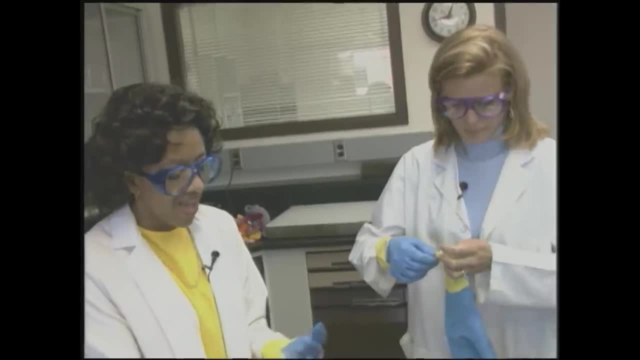 some demonstrations of some mixtures and solutions, What you got. Okay, Let's start off and do a mixture. What's a mixture? Mixtures are things that we can separate easily. Yeah, Now I've done some mixtures at home with like food, salad and. 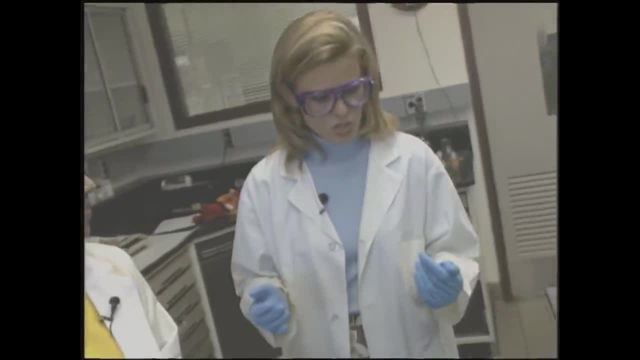 things like that. Now, what kind of mixture can you do here in the lab? Let's do a mixture of. The first one we're going to do is a real easy one to separate. So let's do a mixture of some charcoal and water. 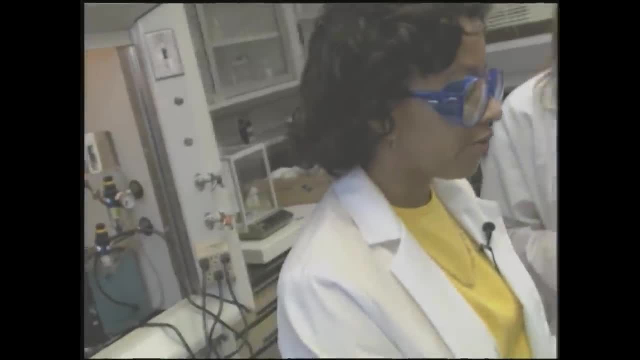 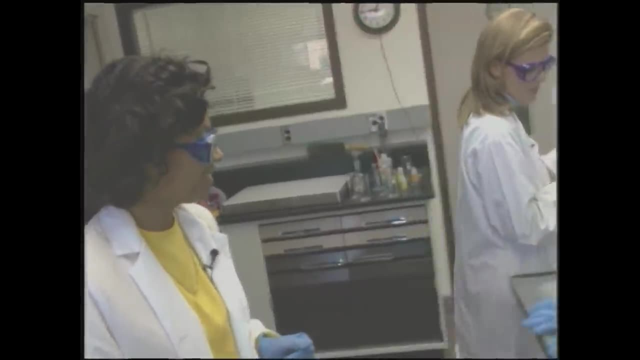 Okay, So Let's start out. You want to get me some water, Water, Sure, Using a beaker here, Right, No graduated cylinder, What is it? It's a beaker. That's a beaker. It's a beaker. 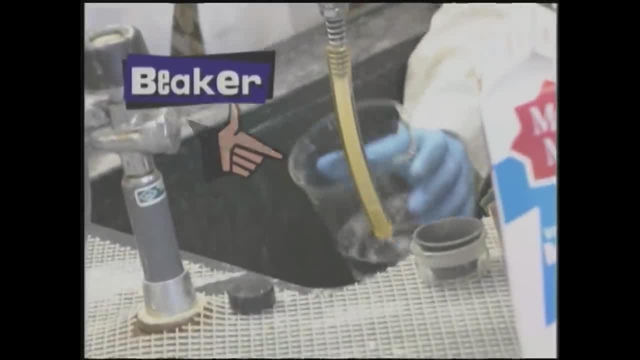 That's a beaker, Okay, So we're going to start out, Okay, And do a mixture, And this black stuff is. This is activated charcoal. We use it to take the color out of things. It's the same thing you use on your fish tanks. 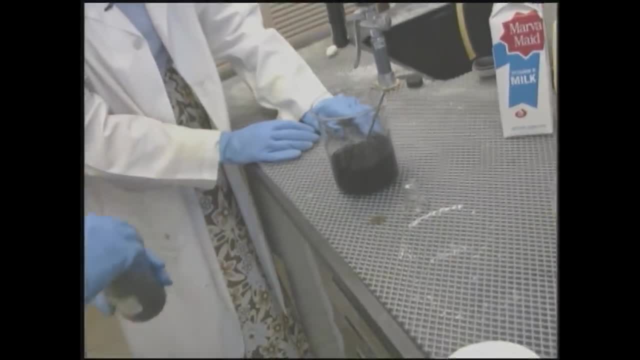 Oh, Okay. For filters on the fish tanks: Okay, But not charcoal like for a grill. No, Okay, Okay. One of the things that we know about mixtures is, if we let them sit long enough, they will settle out. 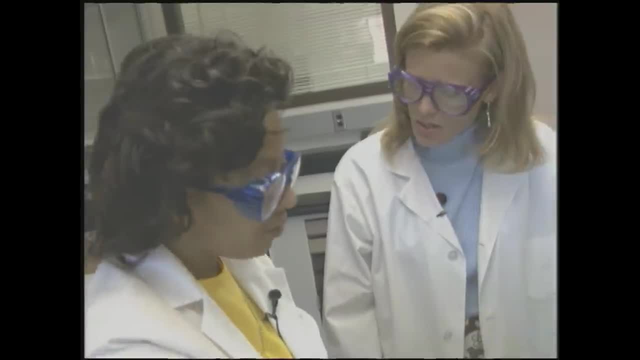 Yeah, And if we let this sit long enough, it will settle out. Now we're going to cheat a little bit and go a little faster. We're going to filter it, And that's another definition of a mixture. All right, 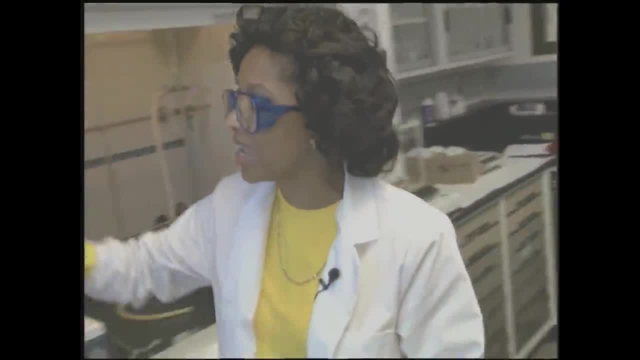 It's something that we can filter. We can do this in the lab, Not at home. That's right, All right, And what we're going to do here is we put a piece of filter paper. I've put a couple of pieces of filter paper inside of our 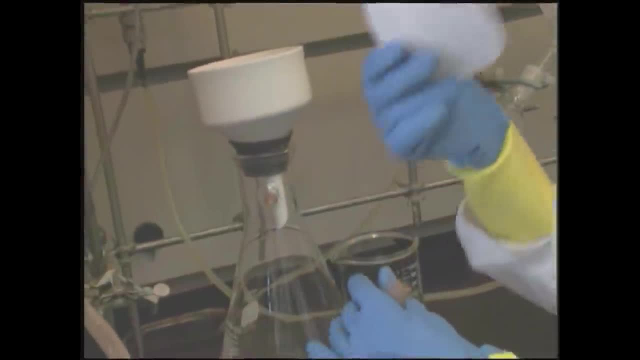 filter, All right, And you're hooking up a tube to it, Right, And this is our aspirator, And the aspirator just pulls a suction on it And let's filter- our solution. You want to do this Sure? 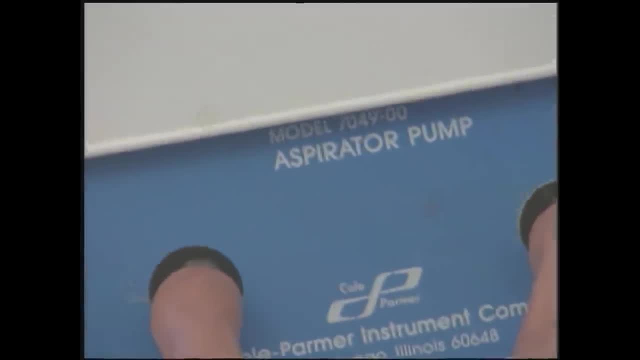 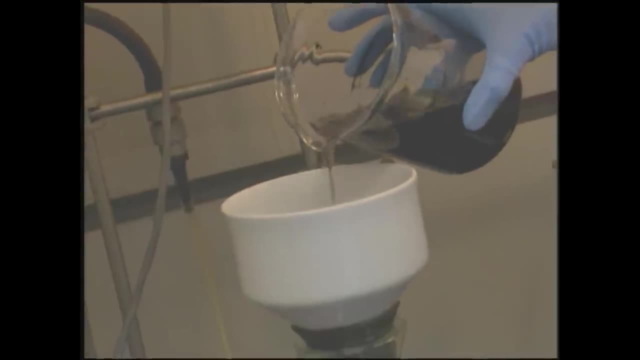 Okay, All right, Right in the middle, doctor. Yeah, You can just fill it up Pour it on in there. Okay, All right, Now we're going to filter. Okay, All right, All right, All right. 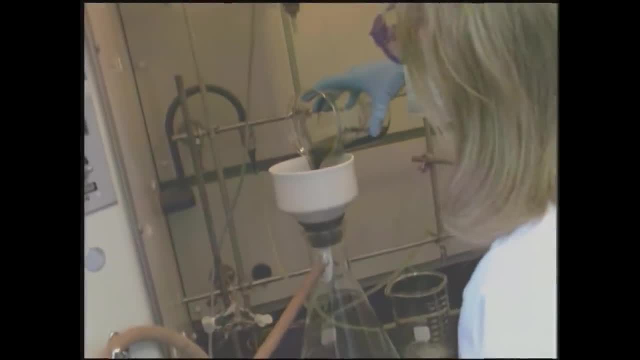 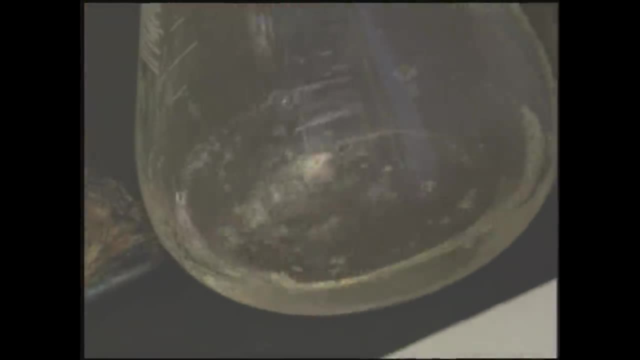 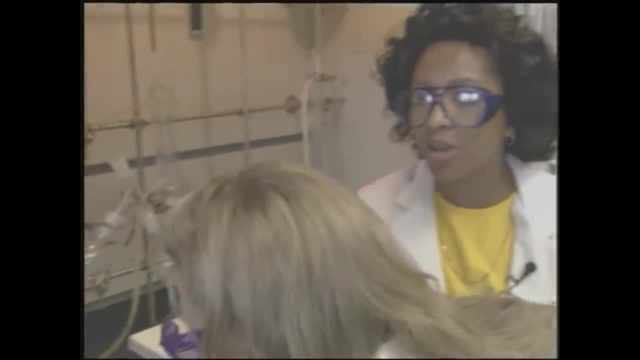 That's right. I don't know. That looked pretty mixed up to me. I don't know. We'll have to see what happens. Well- Now, if you look through in the bottom, you see that we've got the clear water has come through. 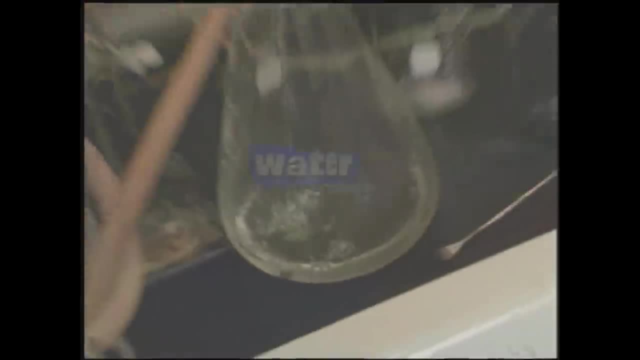 That's the water that I got from the spigot. That's right Now. this mixture is very easy to separate- And that's one of the definitions that we use for mixtures- And then we'll have the charcoal left in the. 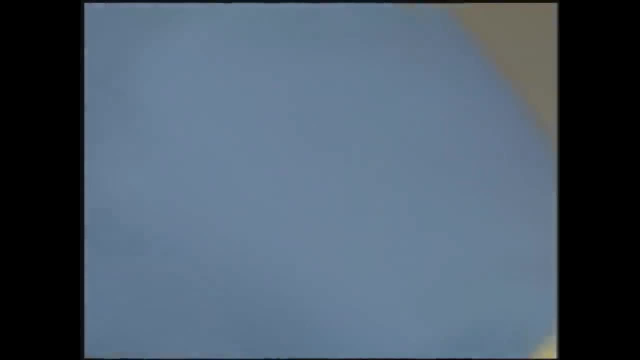 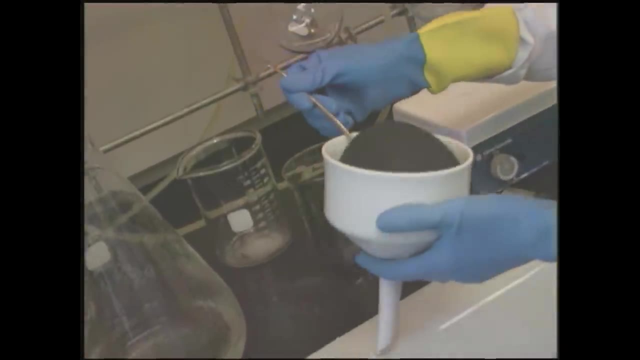 filter, then if all goes well, That's right. And now, if we take our filter off, you'll see that we left with our charcoal. You want to grab that? Yeah, That's amazing. It looks just like the stuff you got right out of the bottle. 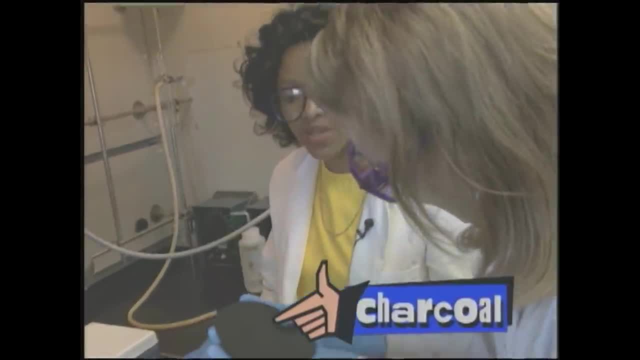 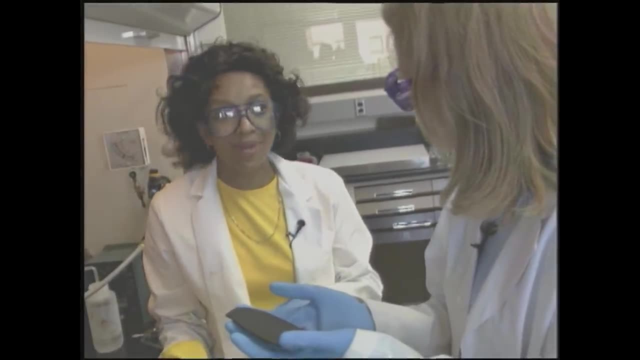 That's right, That is great And it's dry, And it's nice that you had mentioned how things look, And oftentimes we think that when things look the same, that they are the same, And I'd like to do an example where you have something that looks the same but it really isn't the same. 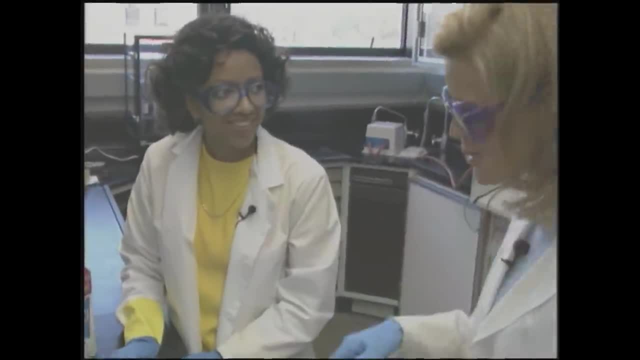 Ooh, Okay, Interesting, Because I love how that aspirator worked. That was great. You totally separated that mixture- That's right- Of charcoal and water. That's great. Okay, what else do you have for me? Okay, now we're going to make another mixture. 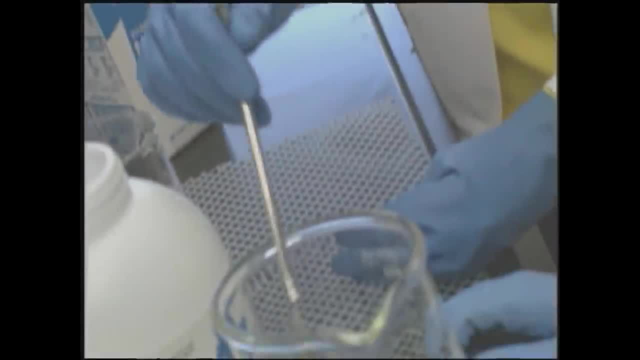 And I guess the main difference in this. now we're using what we call sea light. It's basically a sand, But when we mix it up now it makes a white solution. I'm going to let you mix that up, All right. 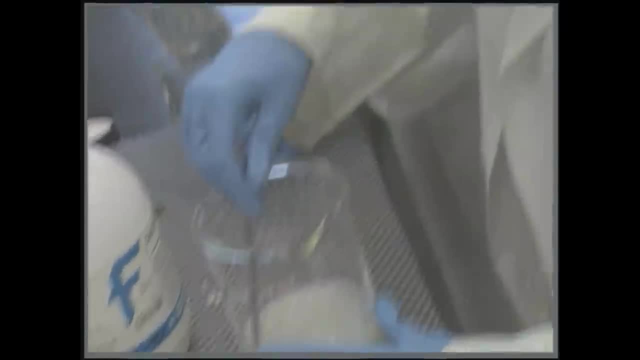 Mixture here That's a mixture of sand and water, Because it's not completely dissolving. then That's right. Is that right? It looks like it is. If you look at that, it kind of reminds us. it looks a lot like milk. 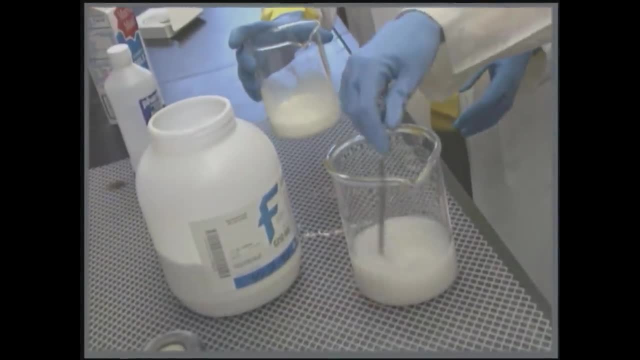 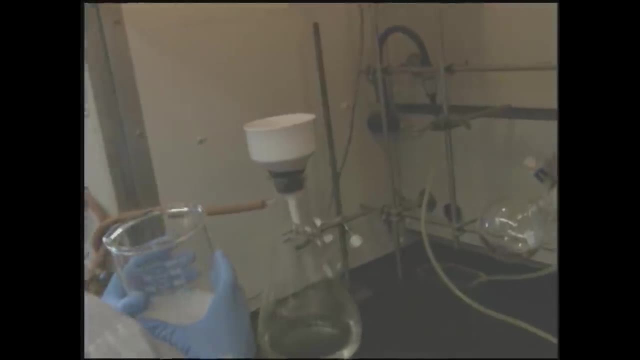 And if you think, if you put it in, we've got two white solutions here. All right, Now let's look at the difference And what happens when we filter these, And we'll decide if it really is a solution or mixture. 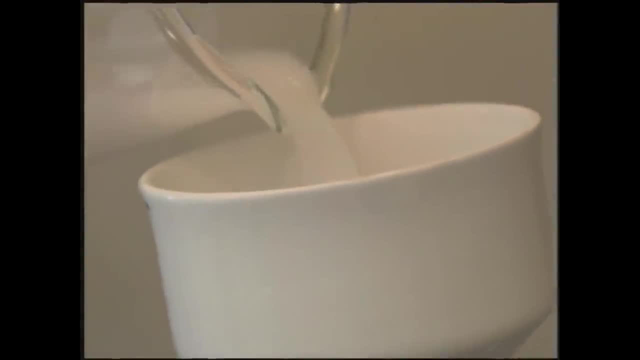 So we'll see. We don't know Mixture solution. We know it's a mixture, right, But we don't know if it's a solution. That's right If it's dissolved it would be a solution. If it didn't, it's a mixture. 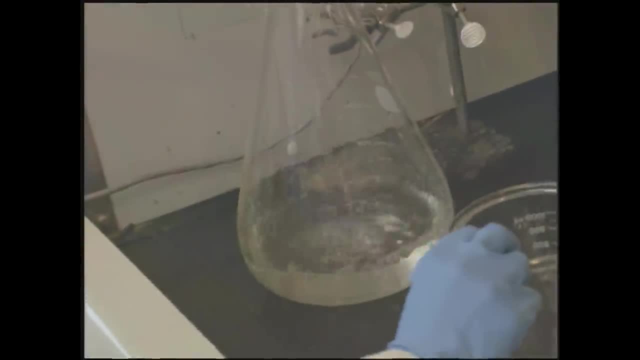 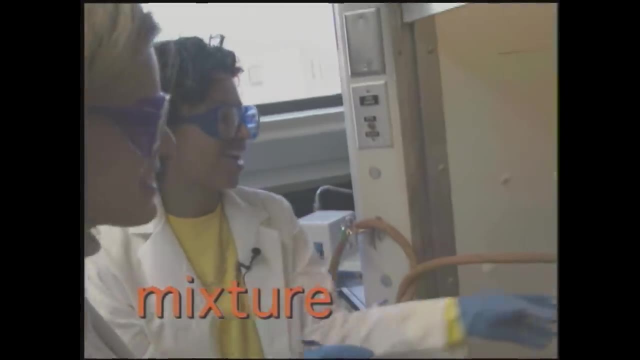 Let's see what happens Now. Jennifer, what do you think this time? Solution or mixture? I'm going to have to say mixture. It didn't dissolve completely, That's right. Easily separated with the aspirator. Yeah, Now let's try our other one. 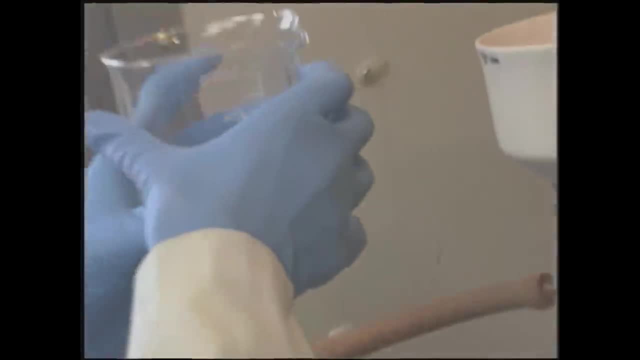 Okay, Let's see The milk. right. The milk, All right, Looks exactly the same as the other one. That's right. Let's see if the results are exactly the same. I don't know. What do you think? 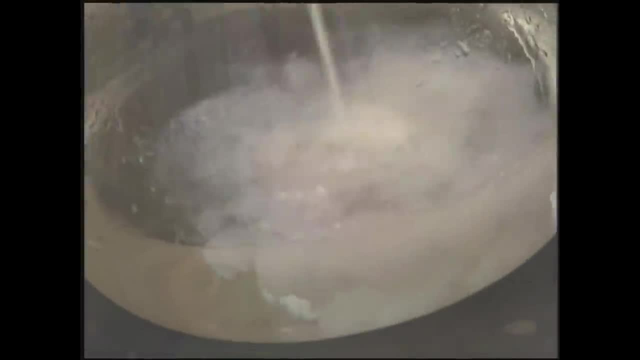 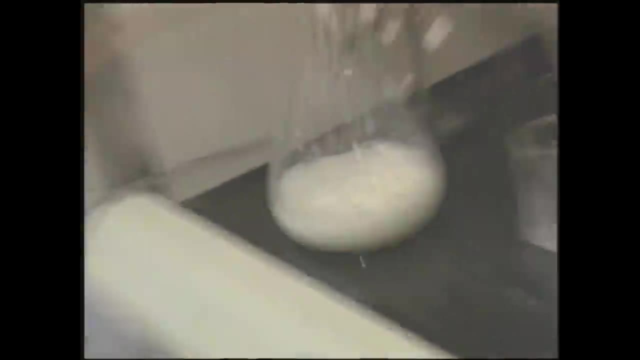 Is it all coming straight through? That's right. There's not going to be anything left on the filter? That's right. And this time, even though it was white, like our mixture of sand and water and milk, we think of milk as the solution. 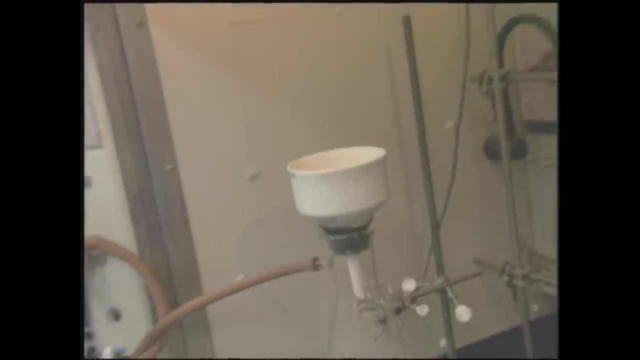 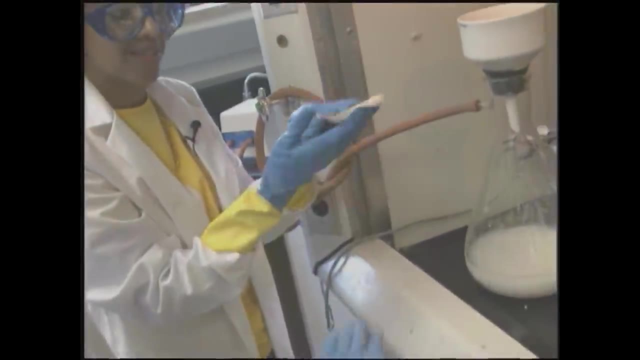 Because everything's dissolved into it and there's nothing left on the paper. Oh wow, That definitely shows me the difference between a mixture and a solution. That's right. Now. let's take our piece of filter paper off and we see: there's nothing there. 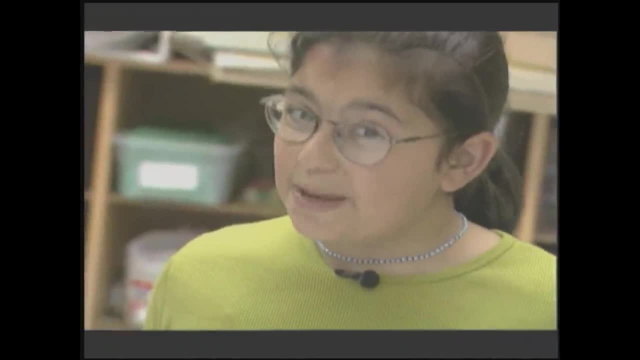 Oh, Just like it was before. So you can't separate the milk? No, that's not true. There are ways to separate milk, but it's not something you can do easily. Okay, It's things that we can do here in the lab. 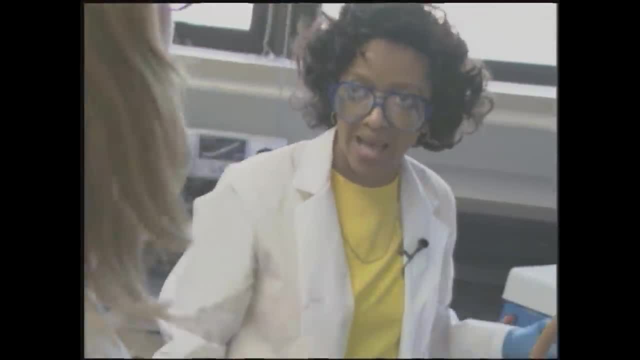 Ah, Not at home, That's right, Okay, Hey, Trish, This is kind of an odd thing to find in the lab. It looks like a piece of chalk. Well, it looks like a piece of chalk, but actually what this is is a magnetic stir bar. 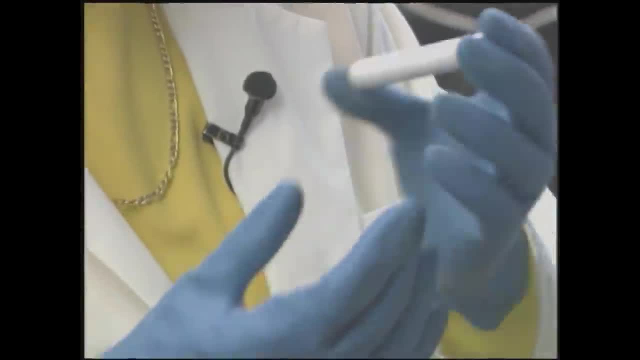 And we use stir bars in our beakers and our flasks to keep things from bubbling over. It keeps things warm, That's right. That's right, That's right. We just stir them like that. Well, no, If you look at this one, it's stirring here. 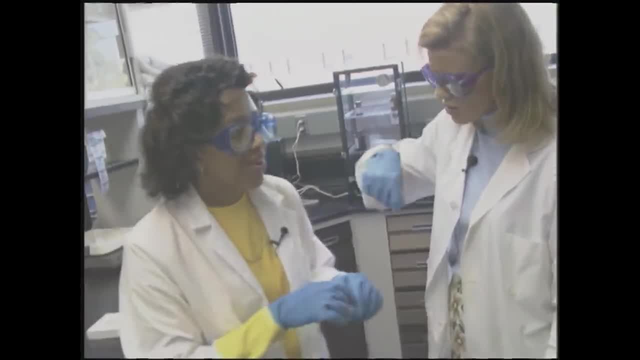 There's a magnet in the bottom, Okay, And this has a magnet inside of it, So it's just two magnets turning, Ah, And it's a way of mixing things, And that's just a smaller stir bar than that one. 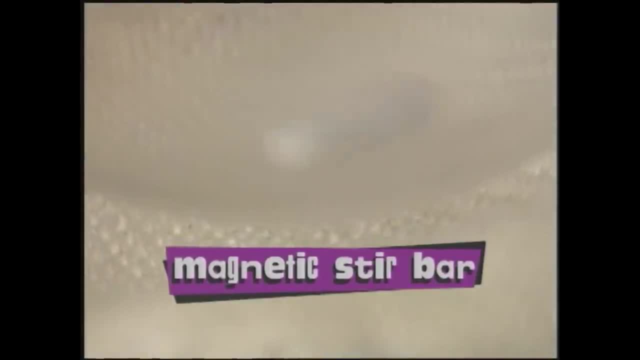 That's right. Well, good, I didn't know what you had chalk in the lab for. you know? No, No, chalk for it. Okay, You're the teacher, That's right. Okay, Now, what you're going to show us is a solution that we're going to separate. 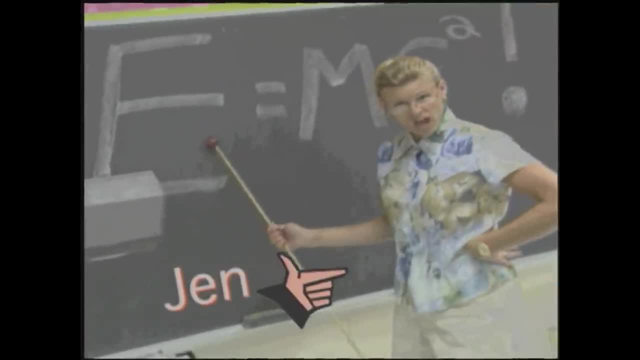 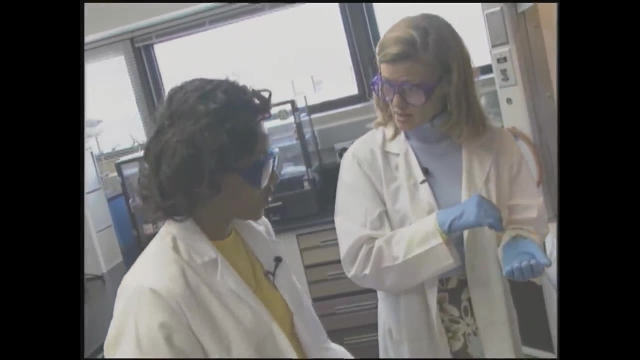 Is that chalk? Yes, Okay. So you're going to show us a solution that we're going to separate. Is that chalk? Yes, That's right, And it's called distillation. That's right, Okay, And that's what this is. 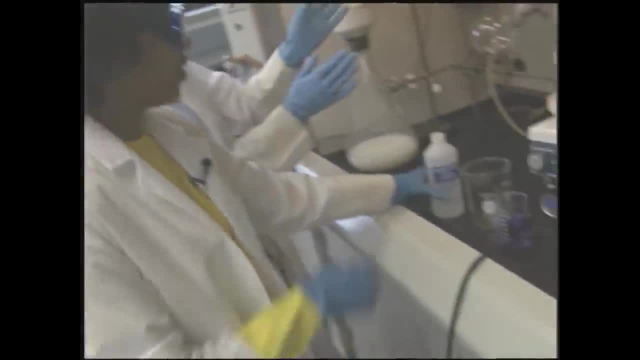 Right. Okay, We've set up a distillation apparatus. This is a simple one, in that we're going to put our solutions in the bottom, Okay. Right here we have a condenser, Okay, Which means, as it boils, it bubbles. 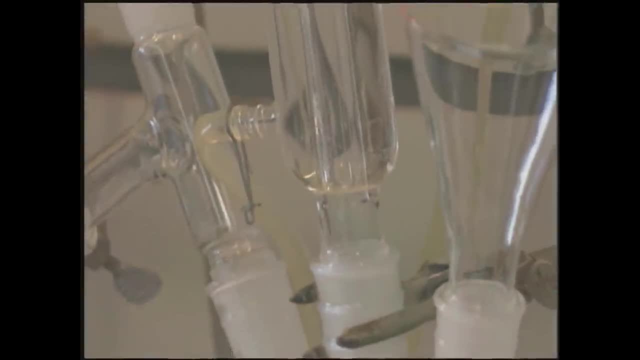 It's going to go up in here, but there's cold water running through it, Okay, So we'll see it condense and drop back down inside. We're going to make a solution of alcohol, Okay, And some water, Okay. 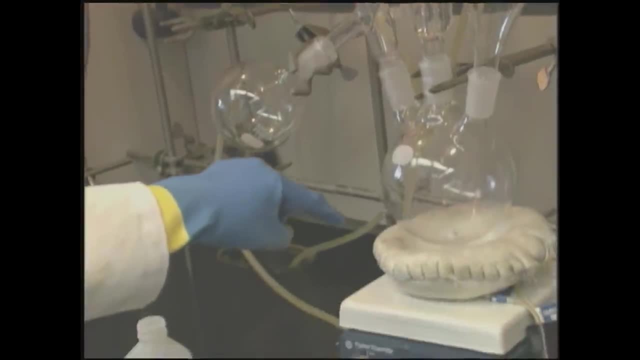 So what we're going to do is we're going to put this in here, Okay, So we're going to put this in here, Okay. So we're going to make a solution of alcohol, Okay, And some water. 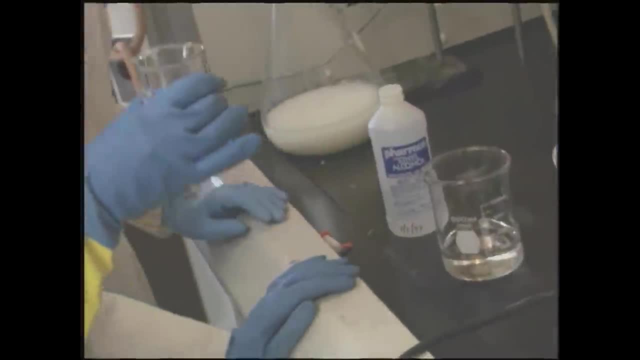 Why is it purple? Because it's my favorite color. Okay, That's why you've got the purple glasses. So now we see that we have a solution And if I filtered this, it would filter through. Yes or no? Yes, it should. 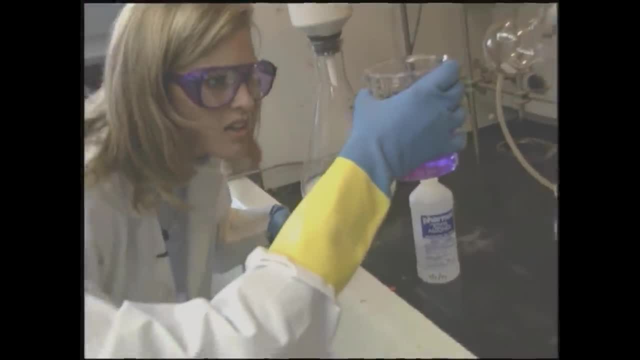 Right. So it would completely go through and there'd be nothing left. That's right. So that's why it's solution. but now you're going to separate it, Right? We're going to show a way of separating these kind of solutions. 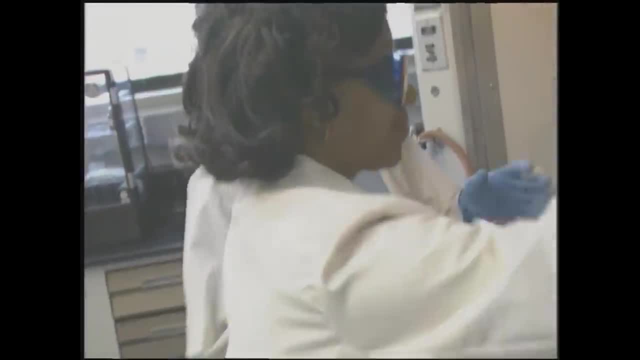 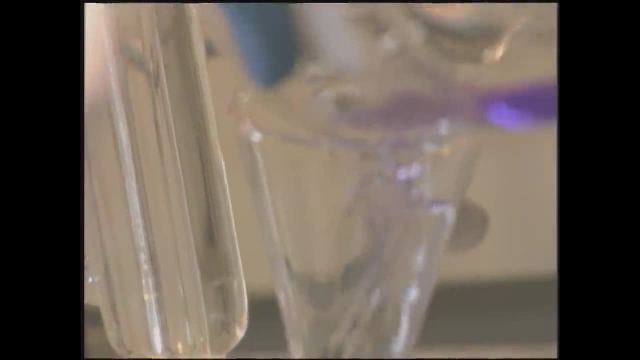 So you just pour it into this, You pour it in through a funnel, Right, Okay? Then take the funnel and put it in here, Okay, So now you're going to separate it, Right? So now you're going to take the funnel out and put a stopper on there so it doesn't. 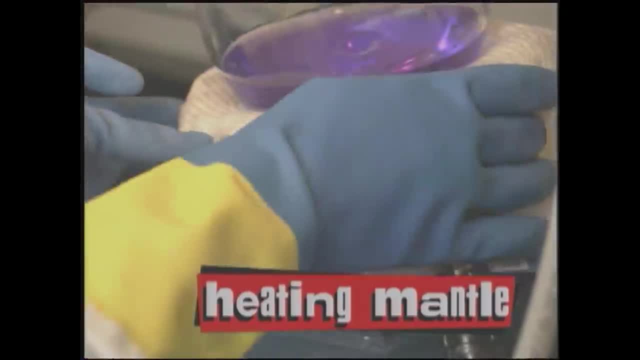 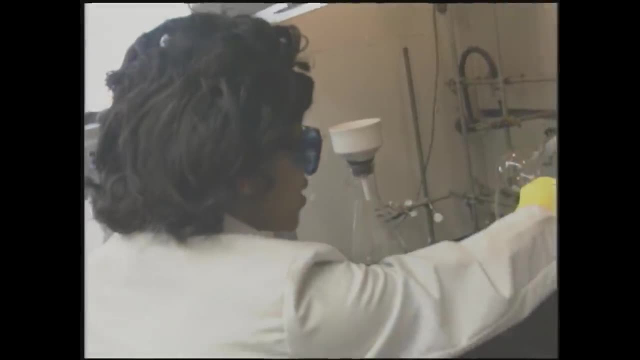 bubble out that end, Okay, And this down here is A heating mantle. I'm just putting this up, So this gets hot. then, Right, Trish, what's happening? Okay, Now we're starting to boil and you can see that the alcohol is starting to drip down. 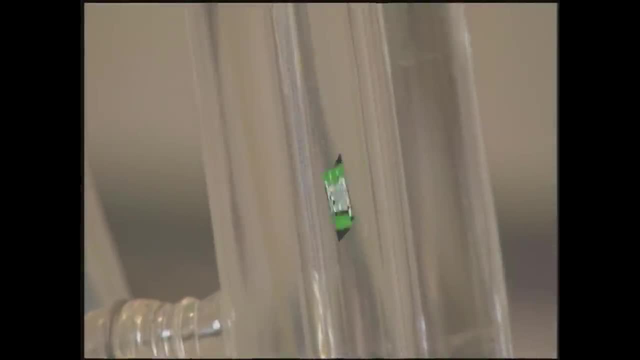 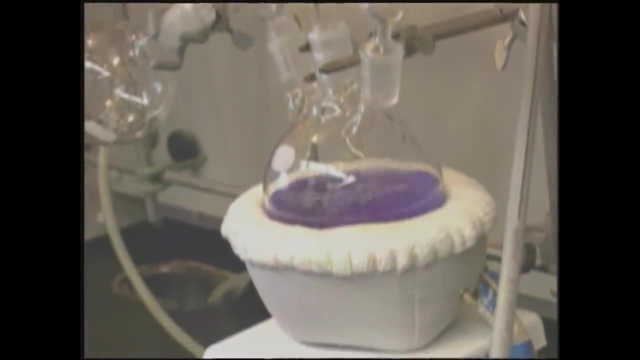 This is actually what we call refluxing. We've got the boiling water and alcohol and the alcohol is actually starting to go up our condenser. Because the condenser has cold water in it, it condenses back and drops back into our flask. 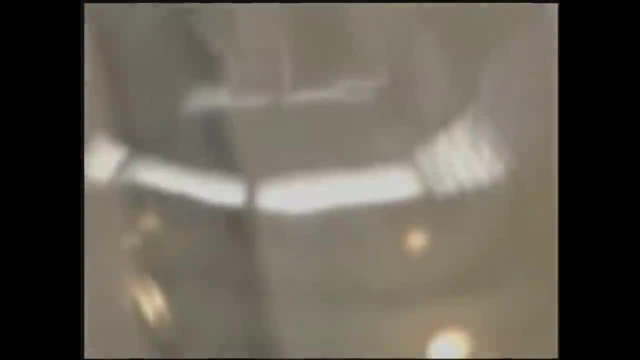 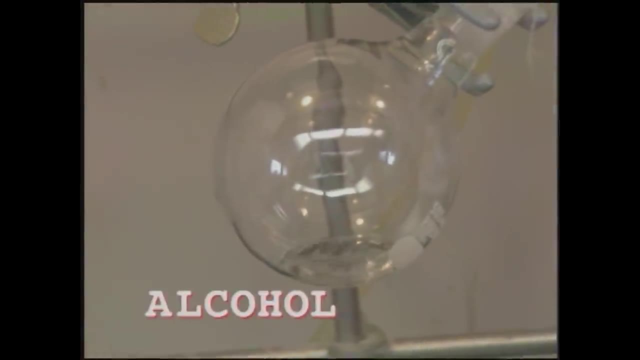 Oh wow. So that's what's dripping back down. is the alcohol? That's right, Trish. is this distillation working here? That's right Now. you'll see that the clear coming over is the alcohol. Oh, It's distilling off. 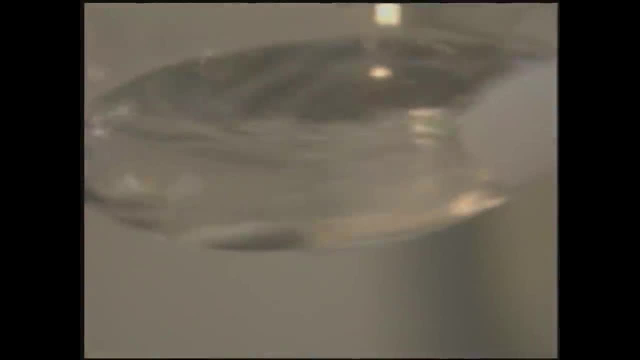 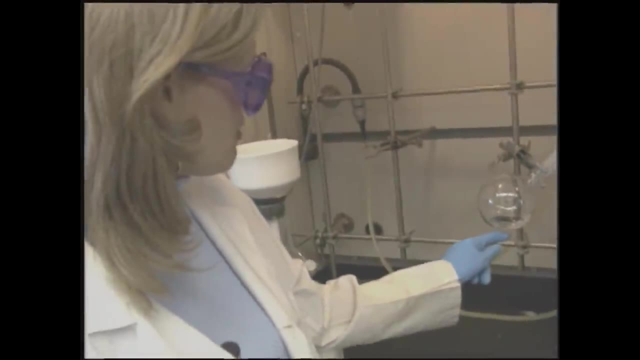 It's collecting the alcohol here. Just alcohol, right, That's right. And we're left with our purple water. So that's pure ethanol, That's right, Trish. thank you so much. We really appreciate this. Well, I really enjoyed having Brain Stew here in the lab to talk about mixed juice and 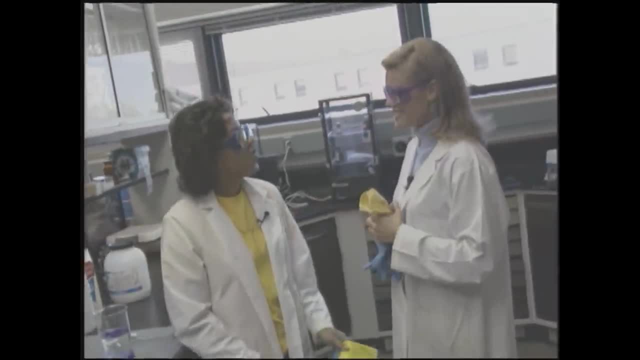 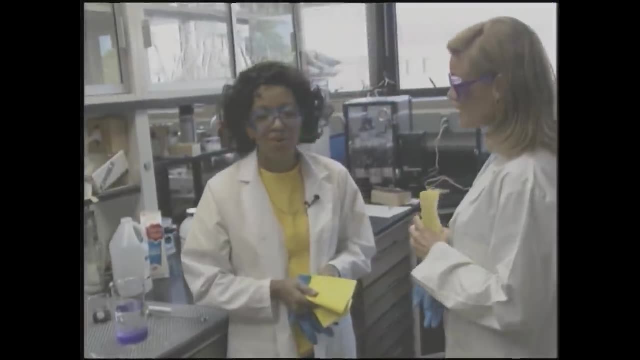 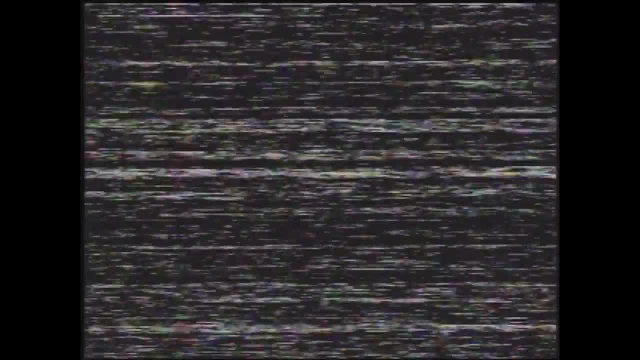 So I can come back whenever we need to do some experiments. That's right for things. Okay, great, Thanks a lot. Okay, I want to thank Dr McDaniel. She did some awesome mixtures and solutions experiments. 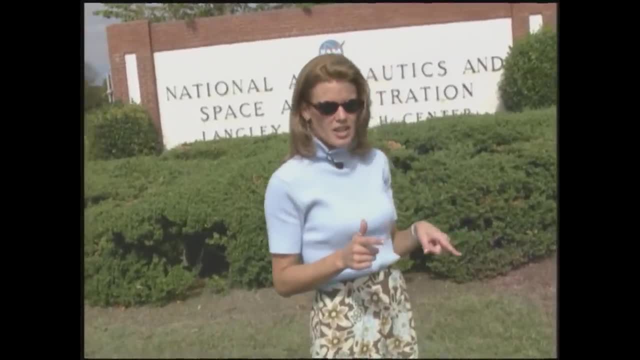 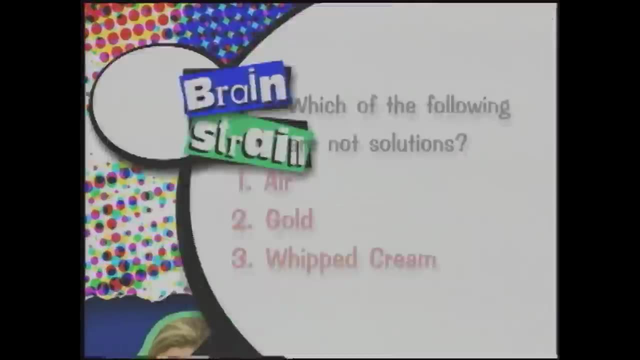 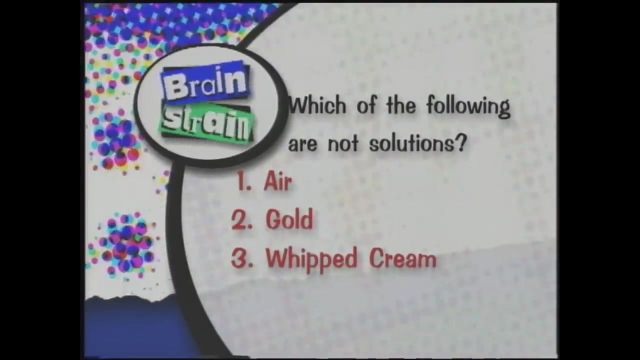 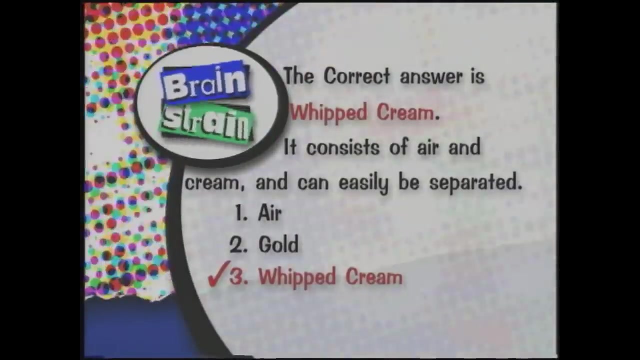 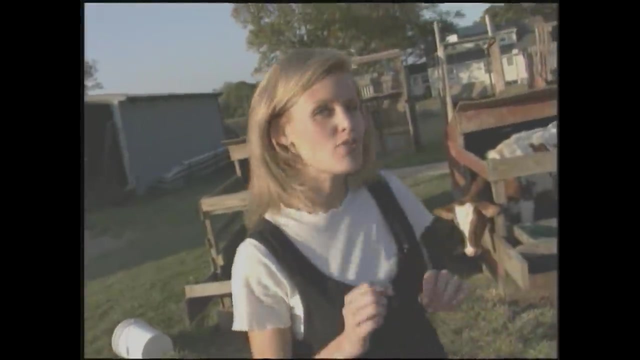 Anyway, guess what? We're off next to Bergey's Dairy. Okay, We've got the cows coming home. We're going over there to see what they have in mixtures or solutions. Hey, I'm here in Chesapeake, Virginia, at Bergie's Farm with Leonard Bergie. 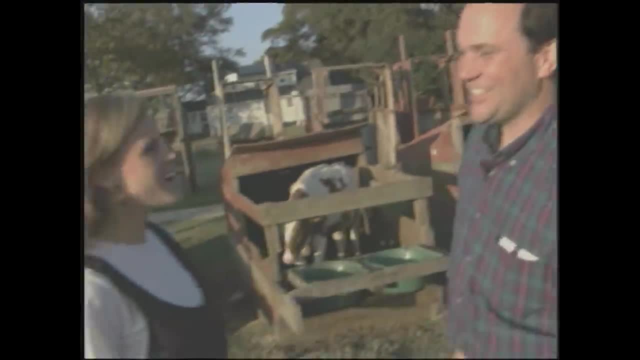 You own this place. Yeah, Hi, Jennifer, How are you doing? I'm doing great. I'm doing great, Great, Great. So excited to be here and find out all the things you do here. Now you have a bunch of cows. 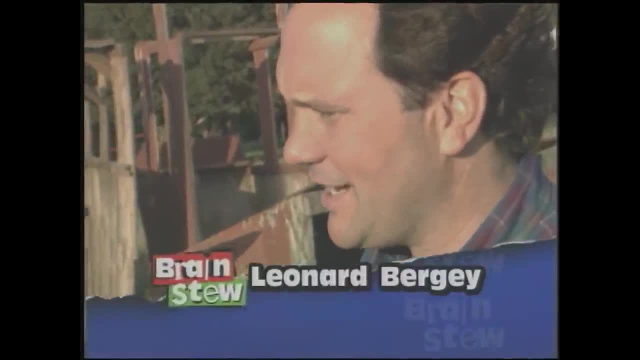 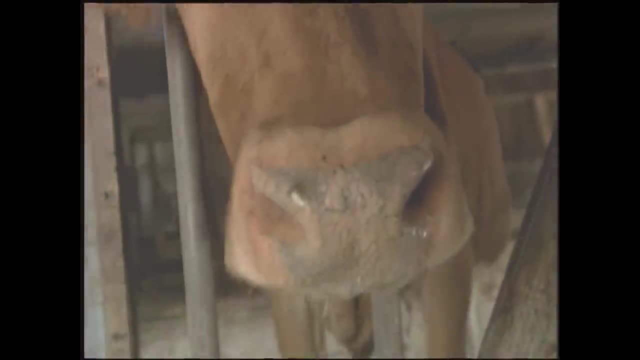 This is your dairy farm. How long have you been here? My family's been here about 60 years Actually. my grandfather started back in the early 30s- Wow- With just a few cows and it's slowly growing now and we're milking about 110 cows now. twice. 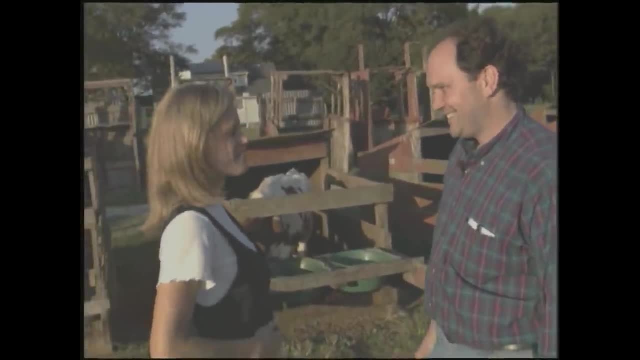 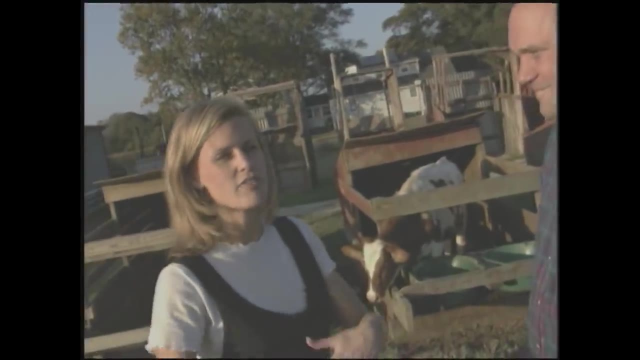 every day, Okay. So you're getting milk every day, That's right, Right. And you get my favorite. you get ice cream every day, right? That's right, Okay, Everybody loves ice cream, That's right, And that's what we're talking about. 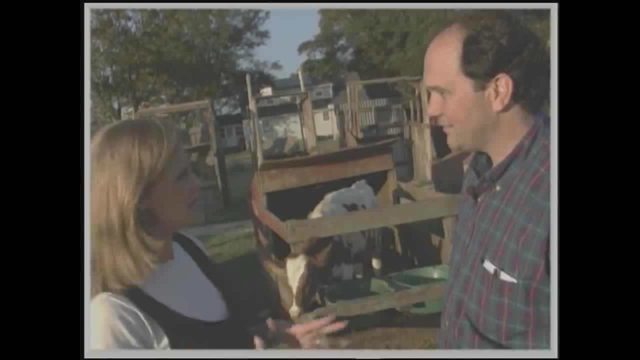 I mean, you know we're talking about mixtures and solutions. I don't want to get off into what my favorite foods are and things, But we're talking about mixtures and solutions. Can you explain to me kind of the process of making ice cream, I mean from the cow? 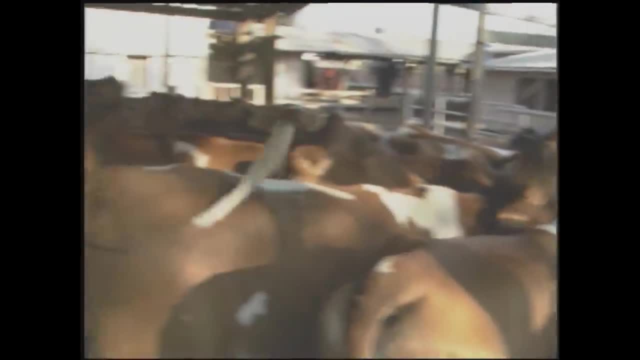 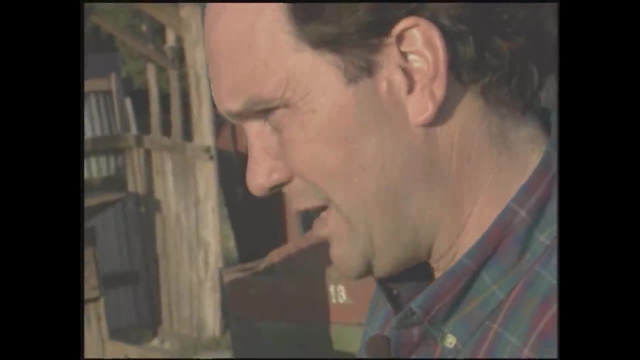 to the finish. How do you get the fresh product? We milk cows twice a day and we get the milk and we actually have to separate it. We separate the skim from the cream and then we use that cream in making the ice cream mix. 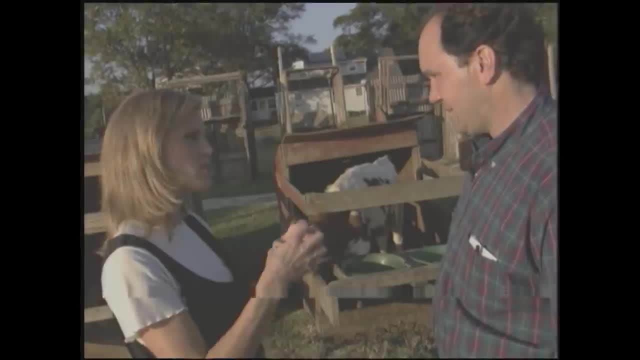 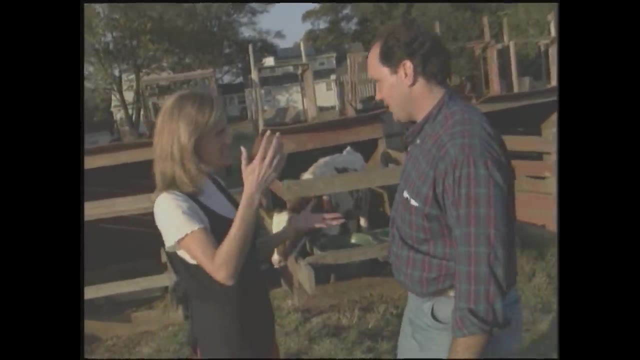 So at that point then, when we separate it milk, at that point it's a mixture. That's right. Just what he said, Exactly He knows. So it's a mixture because it's easily separated. That's right. I guess it's like oil and vinegar. 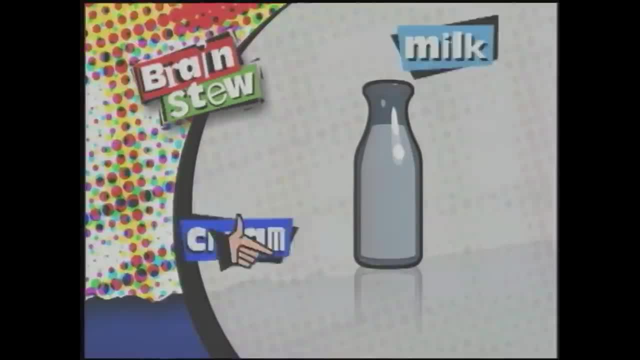 The cream will fall to the bottom. That's right. Is that right? No, the cream actually rises to the top. The cream is lighter, so it rises to the top naturally. Okay, So you've got the cream on the top and all the fat and the 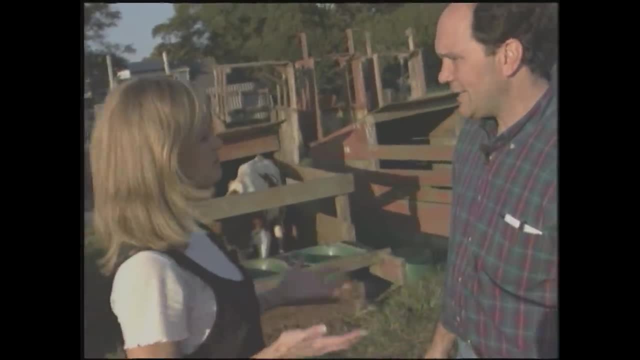 That's right. The skim on the bottom, Okay, And that separates. And then what? That's right, It naturally separates that way, but we have to run it through a separator, a stainless steel machine that will separate it quickly. How does that work? 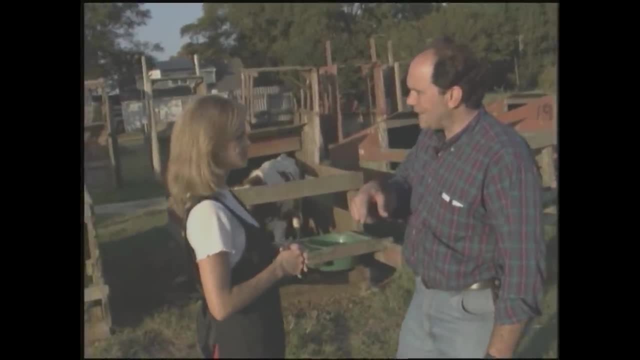 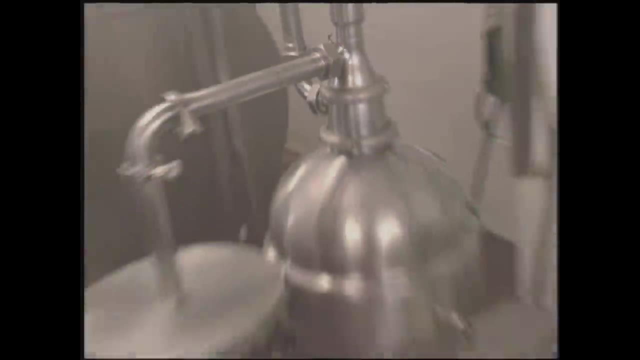 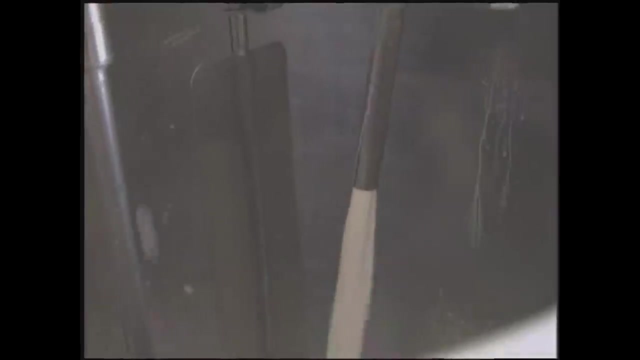 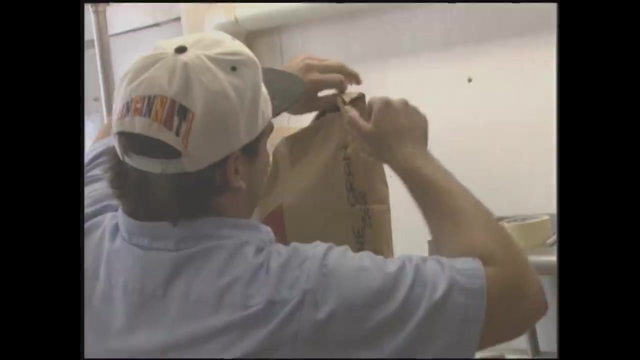 Centrifugal force actually spins it out, so that the cream comes out an upper pipe and then the skim milk comes out of a lower pipe. Oh, that's easy. And so then we take that milk and cream And we actually add sugar, milk powder and a little bit of stabilizer and we blend. 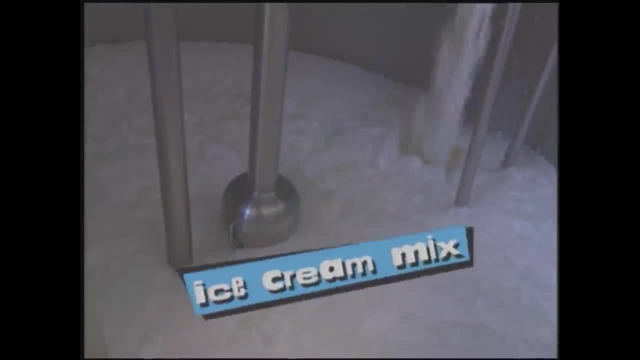 and mix those together to make the ice cream mix. Okay, So when the sugar goes in, I guess it's dissolving into it. That's right. So it's becoming like a solution. now, That's correct. Then we pasteurize that. 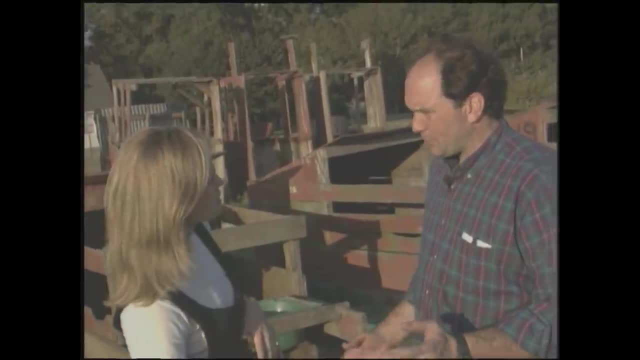 What does pasteurize mean? That means we heat it up to kill the bad germs. It has to be heated up at 160 degrees and held for 30 minutes To kill all the bad germs. That's right: To kill all the bad germs. 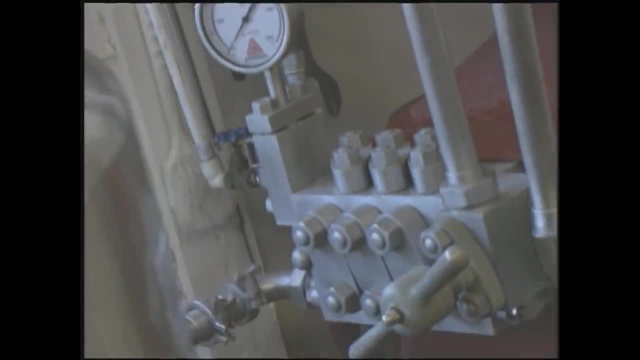 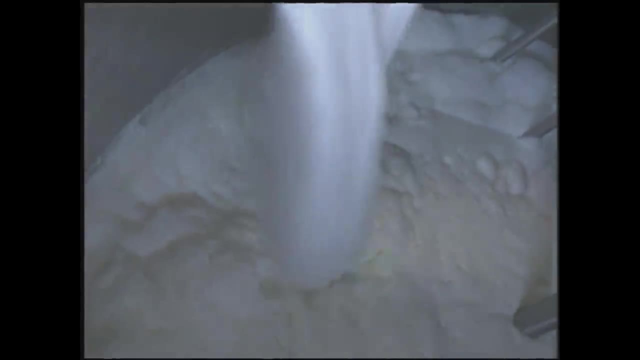 Yes, Okay, Okay, That's right, Okay, And then we homogenize it. Huh, That blends it again. In fact, that makes it even more a solution, Exactly Because it's breaking up things even more. That's right. 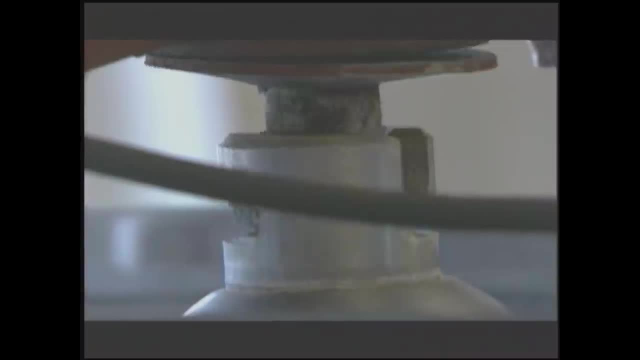 It's making it more and more difficult to separate at that point. That's right. Very difficult, In fact, it cannot be separated. Homogenization: it's pressurized, Is that correct? That's right, Okay, 2,000 pounds of pressure. 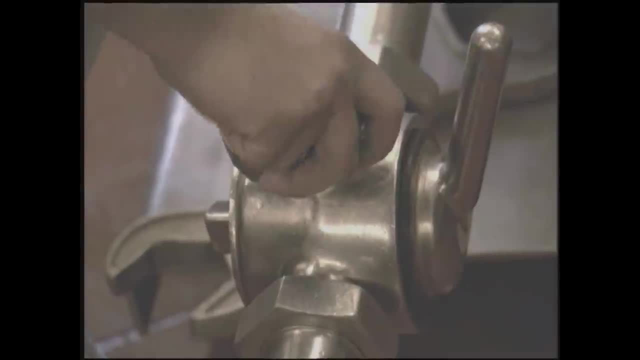 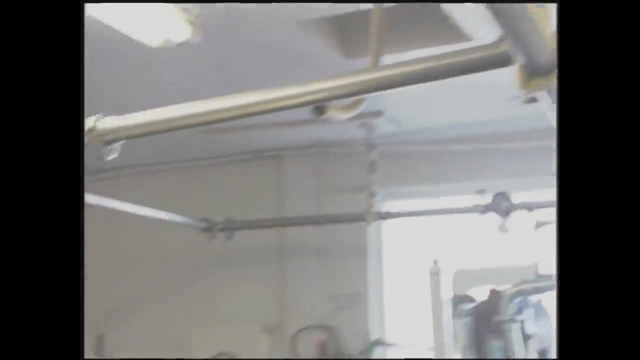 The milk or the mixture is forced through a small valve at 2,000 pounds of pressure, And that breaks it up very small. So it's well, There's no way it's going to be separated, That's correct. And then it goes down through a pipe and up into this big container. 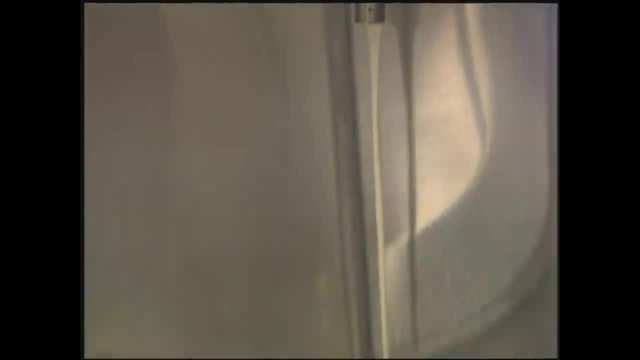 That's right. And what does that tank do? It's cooled down again Down to 40 degrees, From 160 to 40. Boom, That's correct, Boom, Wow. And it's chilled and then stored at 40 until we're ready to freeze it. 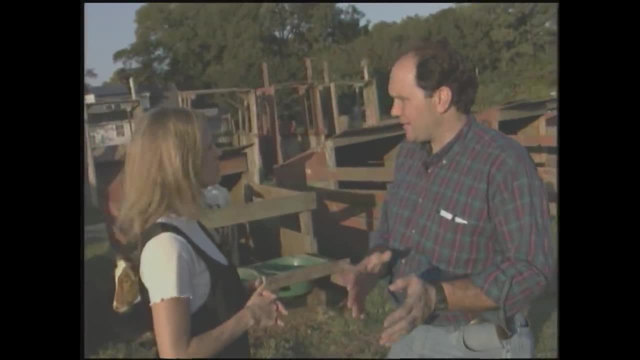 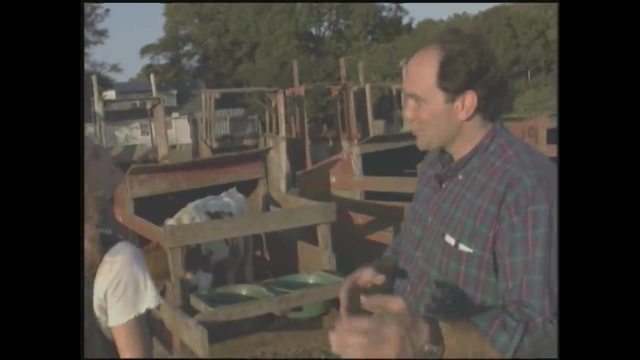 And that's actually where we whip the air in and also add the fruits and flavors, nuts, whatever goes in. Chocolate, Chocolate Strawberry, Oh dear. Well, let's get side here. Triple chocolate, Oh well, no, Oh yum. 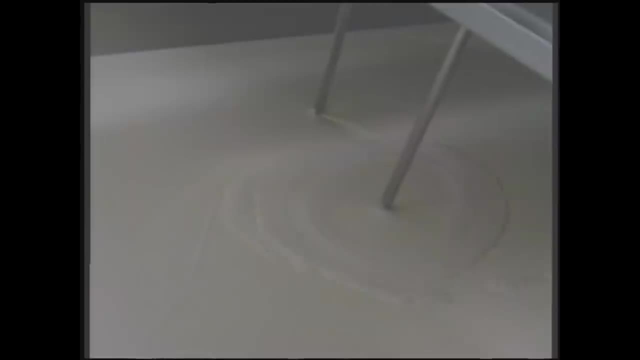 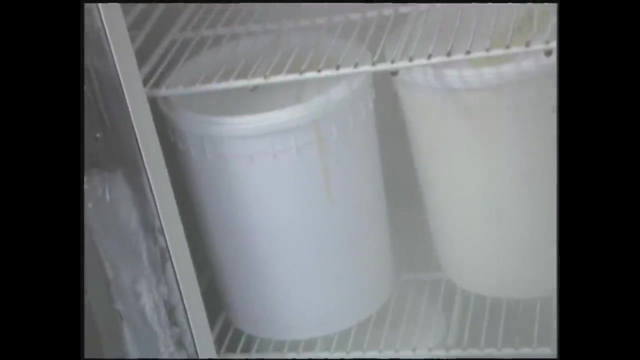 When it's frozen it comes out as a soft serve, Yeah, Sort of, And then it's actually put in a hardening cabinet which is a very cold freezer, blast freezer like 30 below And that freezes it very hard overnight. But it doesn't have to be that cold to store. So we then bring it out, put it in another unit and it's actually stored in a freezer at about 10 below to zero. Wow, And then at that point it's got all the nuts. 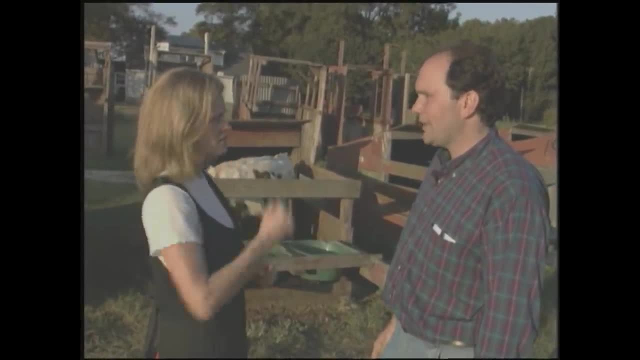 It's got everything in it. That's right. Everything is in it And it's all ready to go. It's all ready to go, Serve it and eat it. Ready to eat, Okay? So how do you milk your cows? 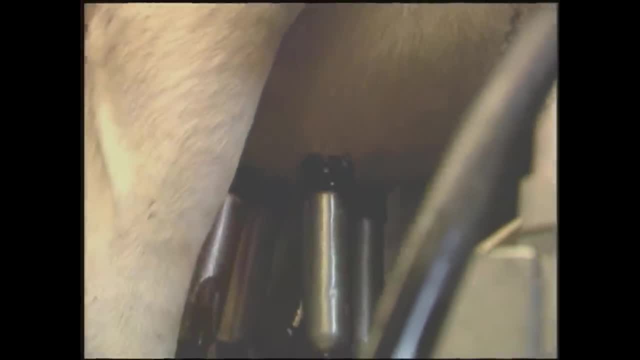 Well, we milk them by machines. Yeah, We actually can bring in eight cows at a time and we milk them with machines. It takes about maybe two and a half to three hours to milk them all, But we have to milk them twice a day. 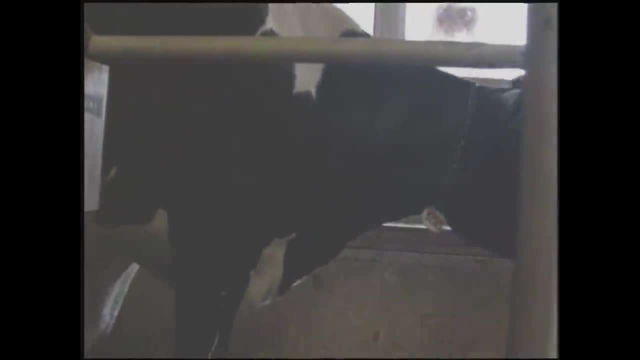 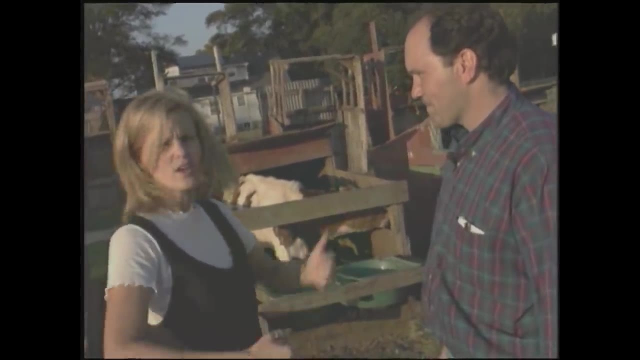 So five to six hours a day someone's milking the cows And you're getting about five gallons a cow. That's right About. And then what happens to the milk? Like, is it in a pail? You know, I always think of this. in a farm, you know, somebody's milking, you know. 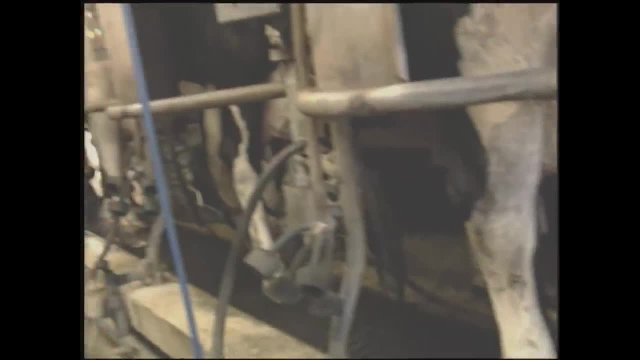 But where you know these machines hook on to the udders. right, That's right. And then where does the milk go? Yeah, It goes through a stainless steel pipe. Okay, It's all stainless steel or glass, Easily cleaned. 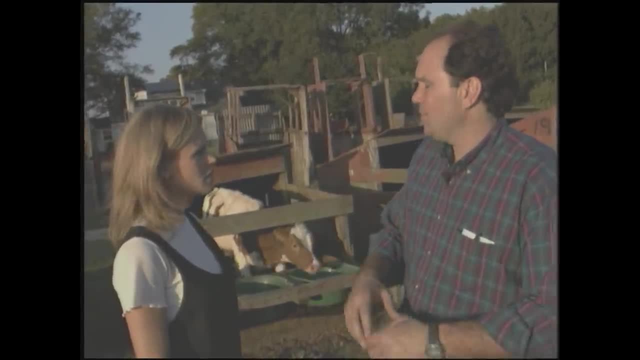 So it goes through a stainless steel pipe into a tank, It's held in that tank And then we actually pump it over into the vat. Wow, And then the vat is where we'll mix in the other ingredients to make the ice cream. 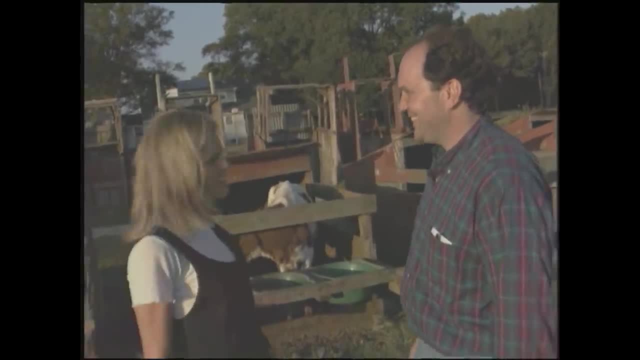 A lot of tanks and pumping, That's right, And vats and you know, cream, All that stuff all around here. Let's go. Okay, Leonard, I'll just talk about all this ice cream and everything. It's great, you know. 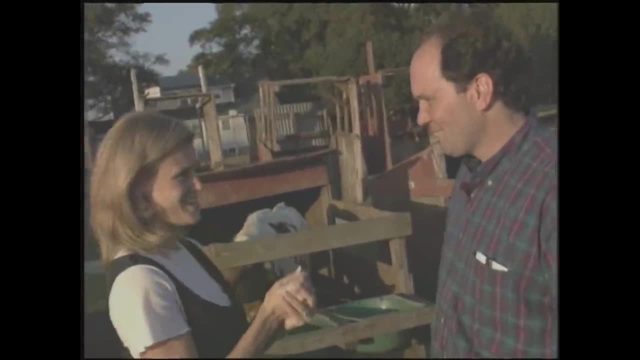 But I want to see the finished product here. I want to see it. I'm getting hungry too, Me too. You want to go get some? Yeah, let's do it All. right, That sounds good. Okay, Leonard, this is it. 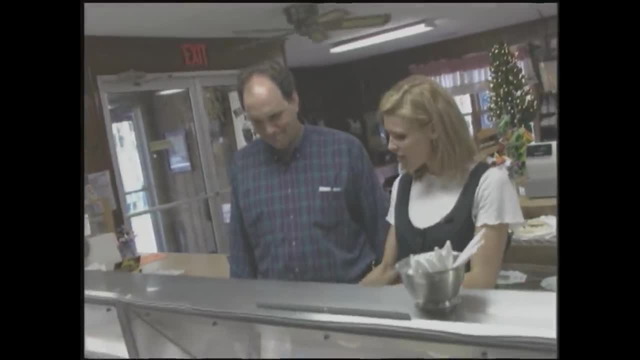 Well, what kind would you like? I'm going to try the toffee crunch. That sounds good. Hmm, that does sound good. I think I'll take pumpkin. I mean, kids, you have got to get your parents to drive you out here to try this. 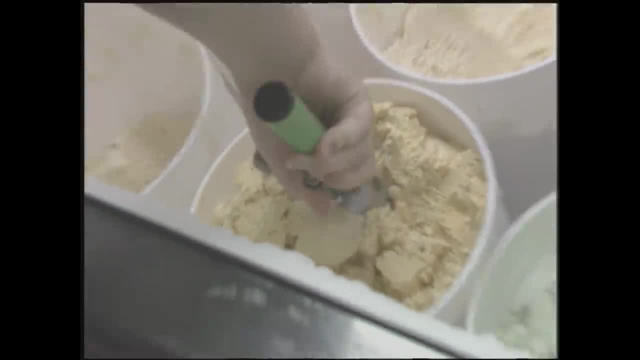 This is the best ice cream I've ever had. It's wonderful. I mean, it came right from those cows out there. This is so great, Leonard, this is awesome. Oh, great. How do you like it? Oh, it's wonderful. 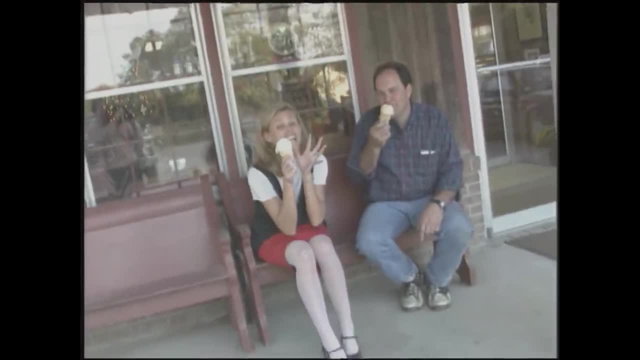 Now listen, Leonard. I'm going to try this. This is the best ice cream I've ever had. It's wonderful. I mean, it came right from those cows out there. This is so great, Leonard. this is awesome. 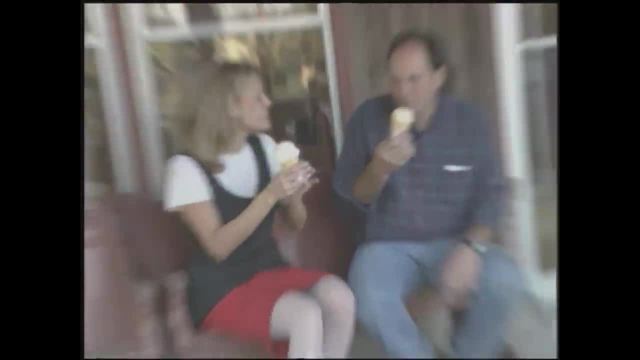 Oh great. How do you like it? Oh, it's wonderful. Now listen. Let me just straighten one thing out here, because I was a little confused, and I don't want them to be confused. When milk comes home and you buy it in the grocery store, you get it delivered. however, 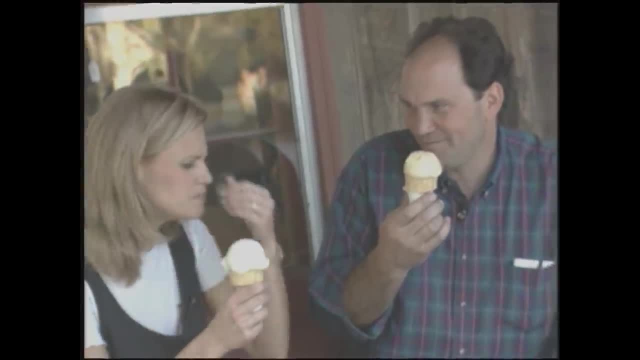 you get your milk. it won't separate easily. The cream doesn't rise to the top, That's right. Why is that? again, Because it's already been pasteurized and homogenized. Okay, I just wanted to make sure. 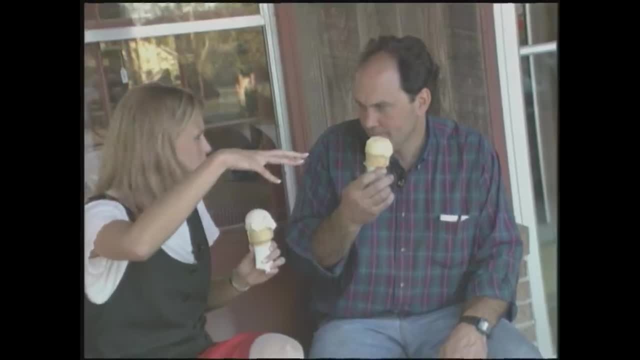 So when it comes right out of a cow, that's when it's easily separated, That's right. So that's when it's a mixture. By the time it gets home, it's already been pasteurized and homogenized. 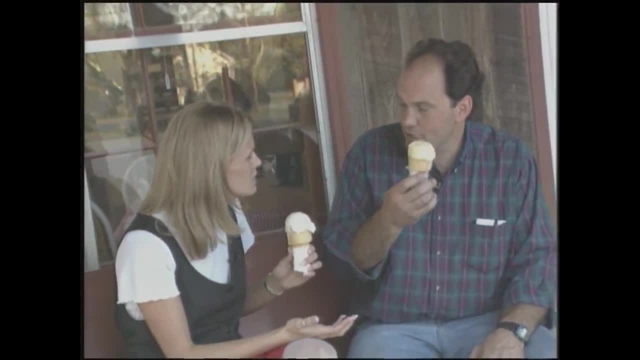 Okay, I just wanted to make sure. So when it comes right out of a cow, that's when it's easily separated, That's right. So that's when it's a mixture. By the time it gets home to the kids and they're pouring in their cereal, the milk is now a 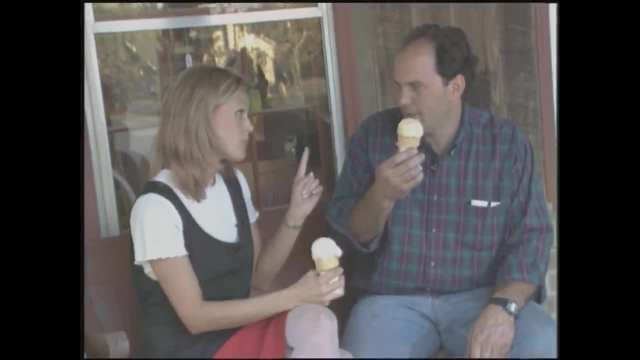 solution at that point. right, That's right. Okay, I got it All right. Well, I want to thank you so much for your time. I know you're busy, man, I'm dripping all over myself here. I want to thank you for your time and letting us come out here and brain stew getting to. 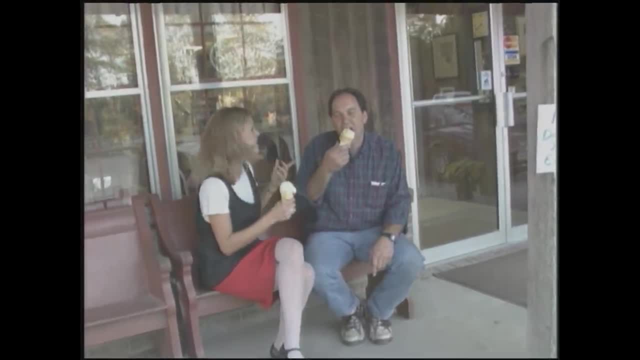 see a little bit behind the scenes of Bergie's Dairy Farm. Cool, Thanks for coming. Thanks a lot, Thanks a lot. Enjoy it Up next. you guys, You don't want to leave, You don't want to leave. 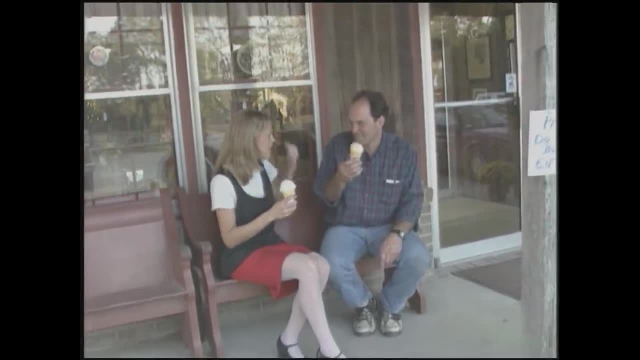 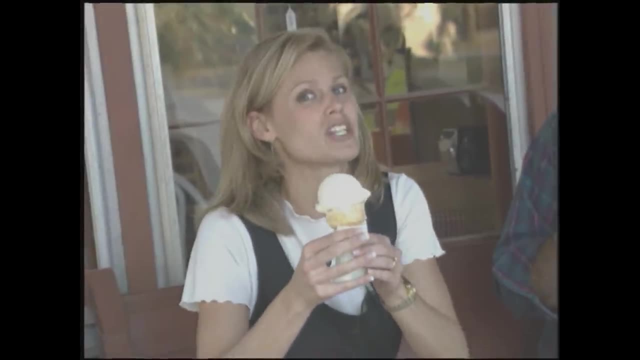 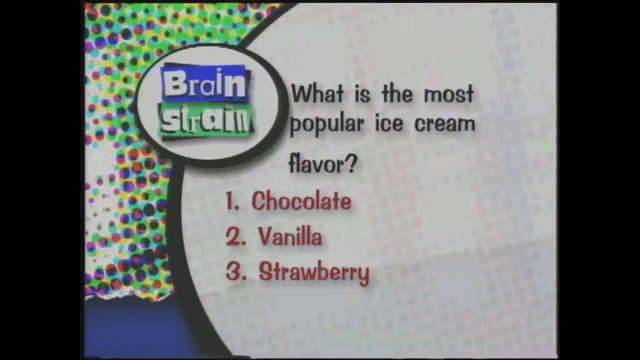 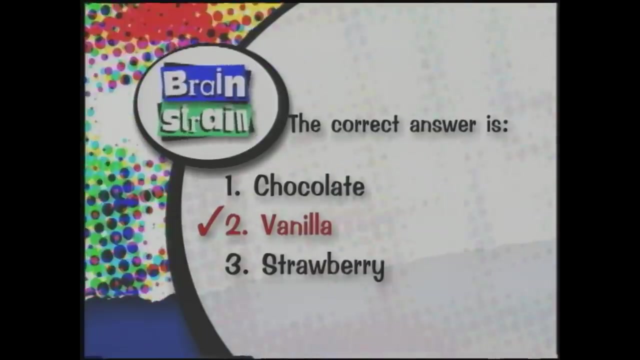 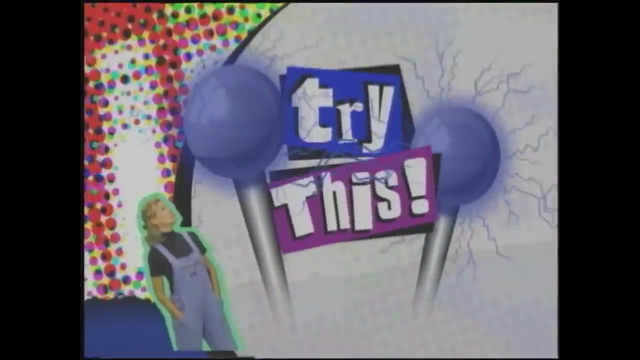 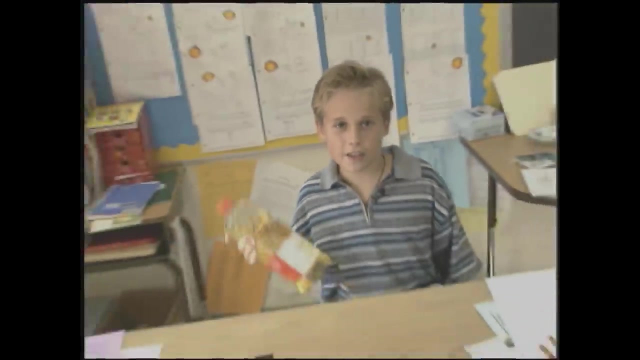 We're not even leaving Chesapeake. We've also got a really cool experiment that you've got to see. This is dripping all over Bye. Here's what happens when you try to dissolve food coloring in oil. Here's what you'll need. 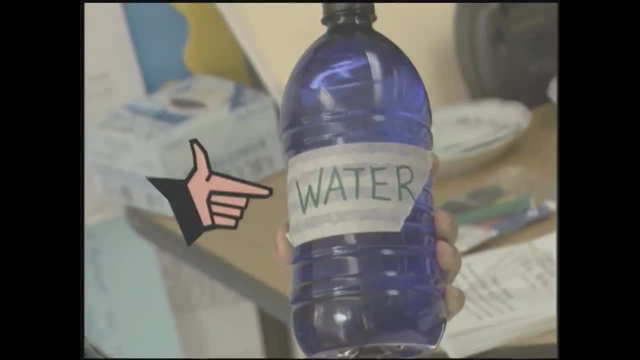 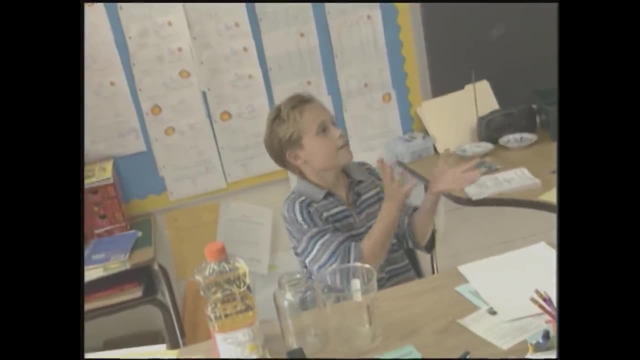 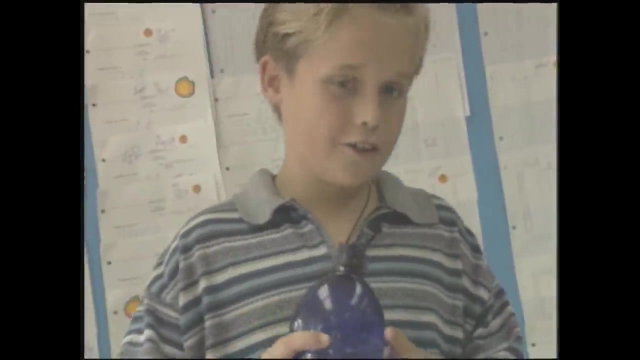 Liquid cooking oil and water, A glass or plastic container and blue food coloring. Here's the procedure: Pour about a cup of water into your container. Slowly pour the same amount of. Slowly pour the same amount of oil into the container. 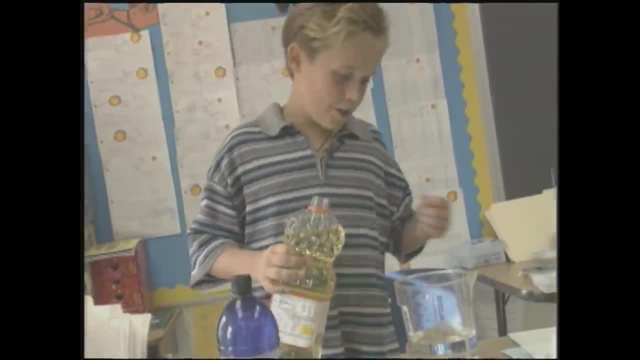 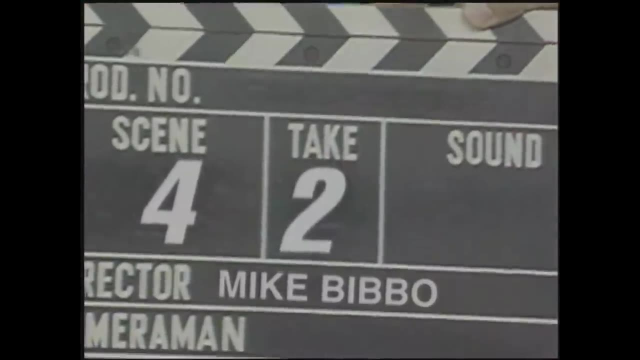 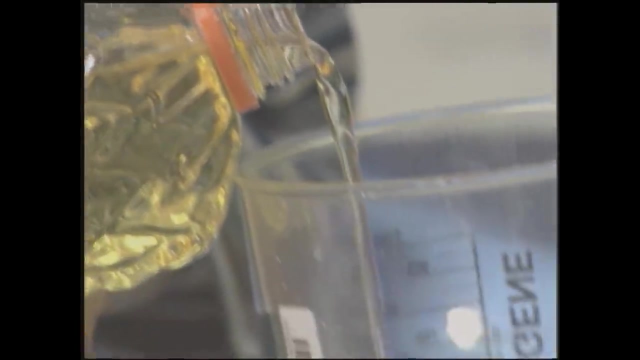 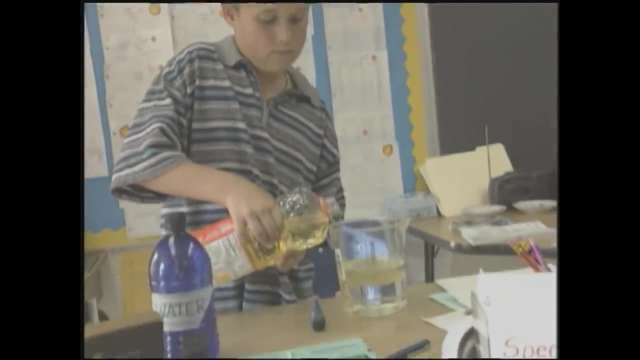 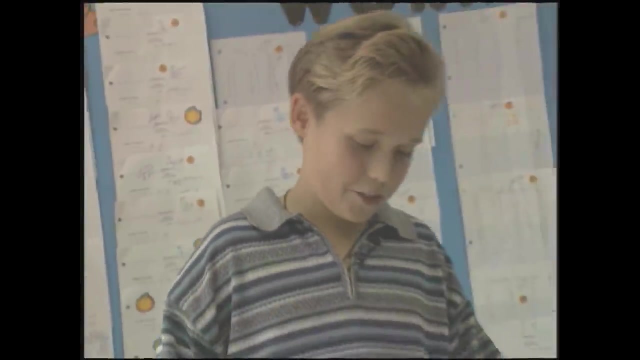 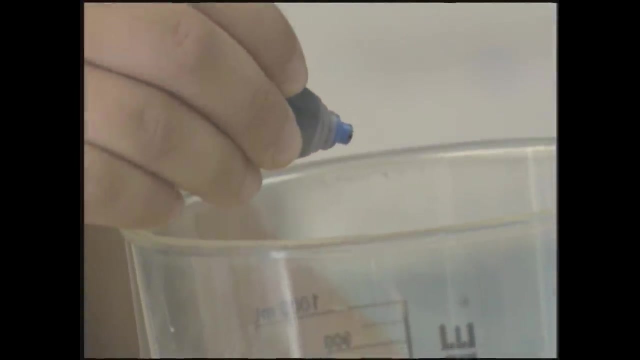 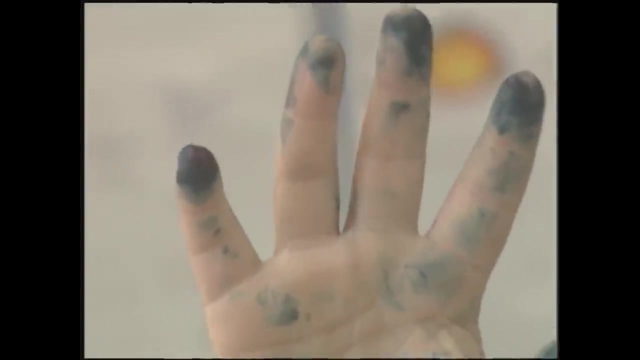 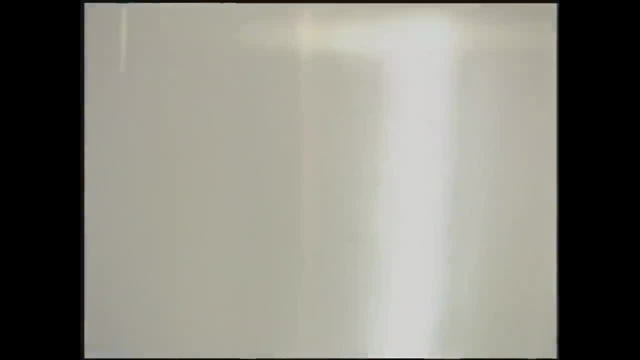 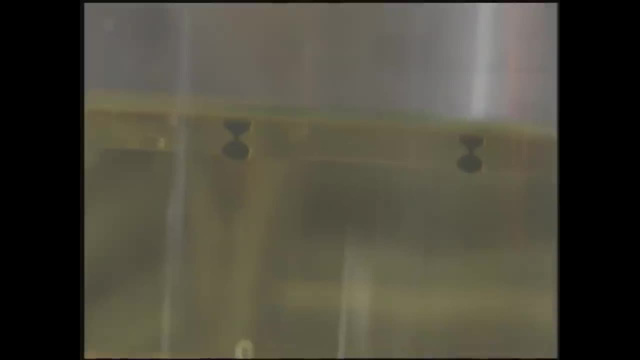 balls sink. If you look underneath, you can still see some of the balls floating in the oil. If you have any balls that don't sink, here's what you do: You take a pencil and you push the ball still floating in the oil all the way down to the water, As soon as 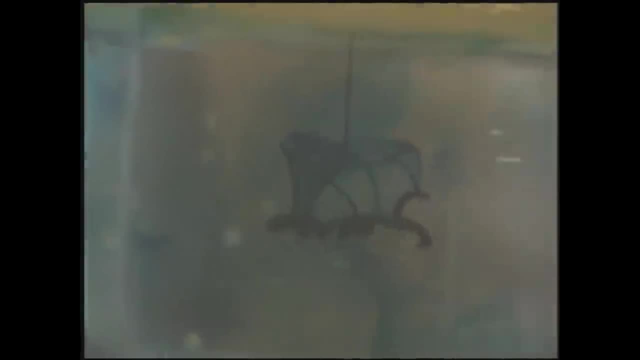 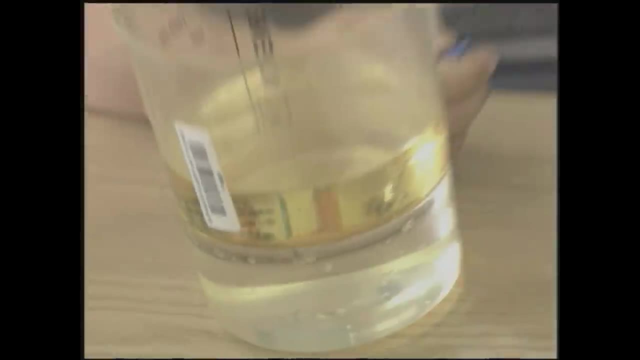 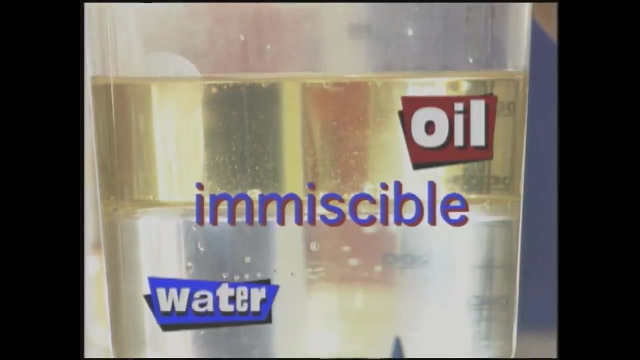 the colored balls touch the water, they immediately break apart and dissolve. Here are the results: Two separate layers form. The oil floats on top of the water because it is lighter, Why Oil and water are immiscible. That means they do not mix and will separate into layers. 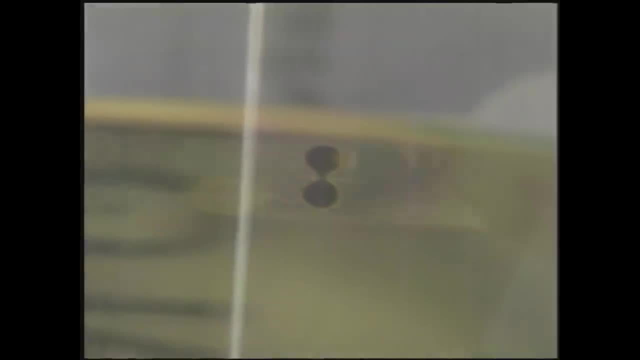 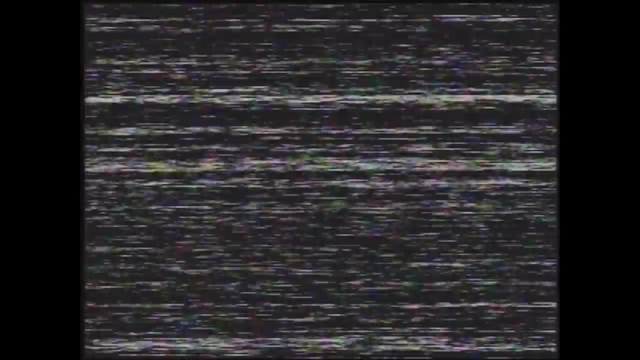 Roof coloring does not dissolve in oil and will float if the drops are small enough. The oil surrounding the balls of color prevent them from touching the water. Pushing the balls through the oil allows them to touch and dissolve in the water. So that's it. 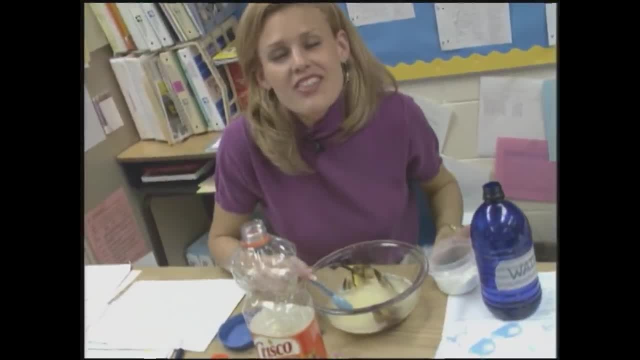 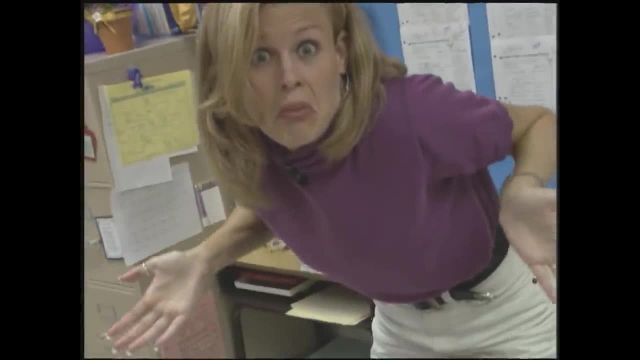 So what is it? A mixture Or a solution, Or both? I want to thank Martha Ann and Margaret at the Central Library in Chesapeake. Those librarians sure know their mixtures and solutions. Think they can figure out what this is. 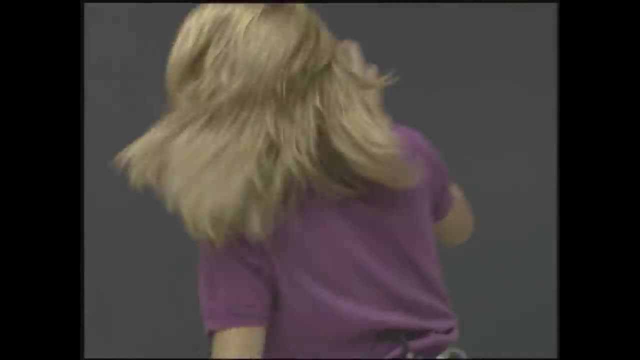 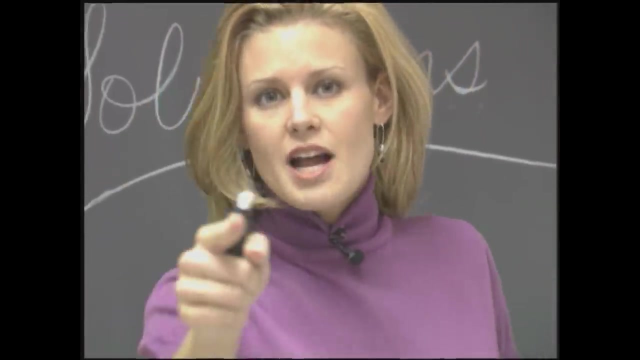 Okay, one more time class. What are we studying today? That's it: Mixtures and solutions. So next time you're out, look around, Look at all the matter. What is it? A mixture, A solution, Or both? 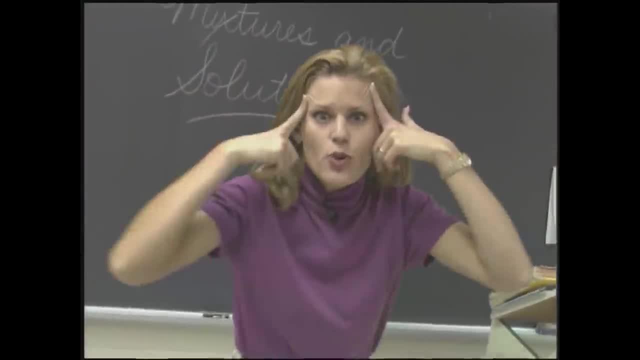 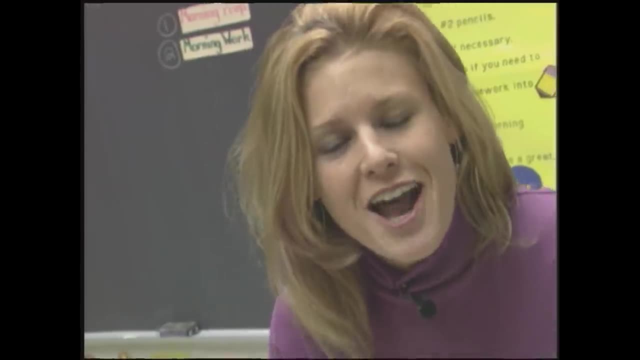 Well, that's our science lesson for this week. I hope your brain is stewing with information about mixtures and solutions. Next week we're- I'm not going to tell you where we're going to be. If you want to find out, you tune in. See you then.